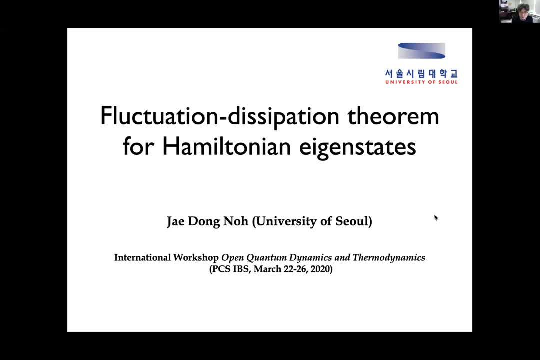 Okay, thank you. First, I'd like to thank the organizer for inviting me to this workshop, So it's very hard to be a part of this kind of event. I think this is a very nice opportunity to discuss physics. Okay, this is my title and my name is Jaedong Noh. I'm in the University of Seoul. 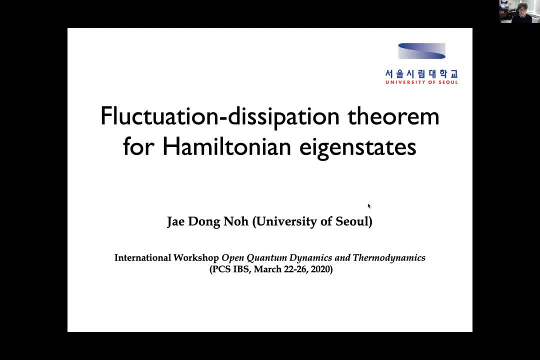 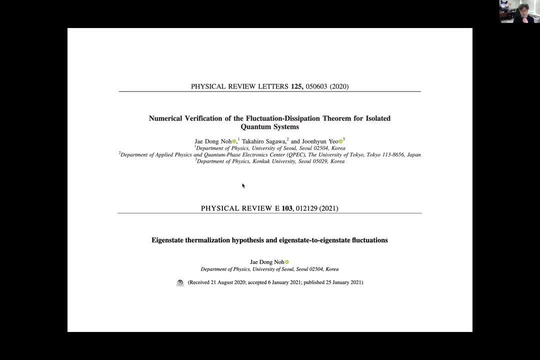 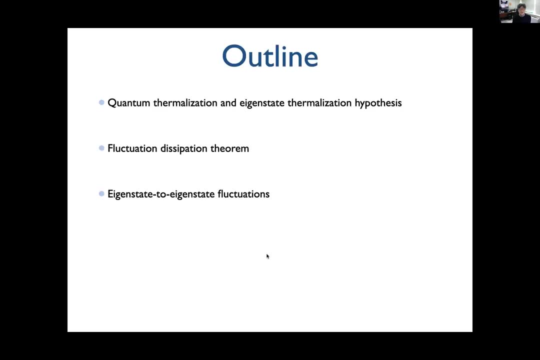 And this talk is based on my recent two publications. One is in PR last year and the other one this January. So this is the outline. So first of all, actually this workshop is about the open quantum system, thermodynamics for quantum system, but my talk is for the isolated quantum systems. So 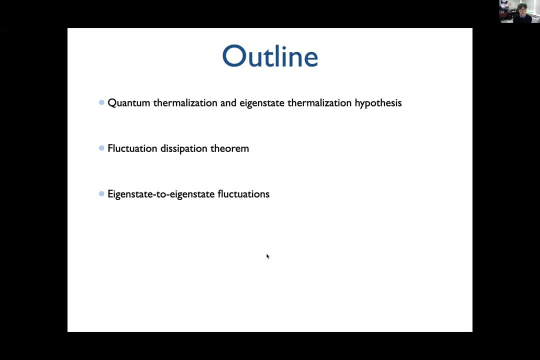 hopefully, I hope, you enjoy this topic too. Okay, So first let me briefly review the concept of quantum thermalization and eigenstate thermalization hypothesis. This is a basic kind of paradigm for understanding of thermodynamics of an isolated quantum system. And then I move to the main part of my presentation. First I will explain the fluctuation dissipation theorem for Hamiltonian energy eigenstate, And then I also try to explain some of my recent research for the so called eigenstate to eigenstate fluctuations. 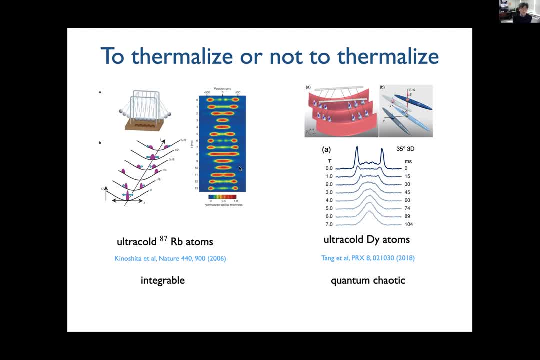 Okay, so what do you mean by the quantum thermalization? In this period we have a big advance in experimental technology in such a way that we can simulate the isolated quantum dynamics. Okay, so, for example, if you prepare some cold atom system in this harmonic confining potential, then you can observe the motion, or measure the motion of the atomic system. 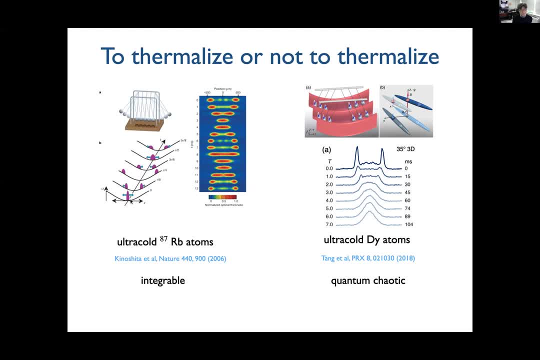 But the only way that we can do it is to study quantum dynamics, atomic cloud as a function of continuous time. okay, So this is a very famous experiment which shows some quantum real, quantum many-body dynamic, real-time many-body dynamics. 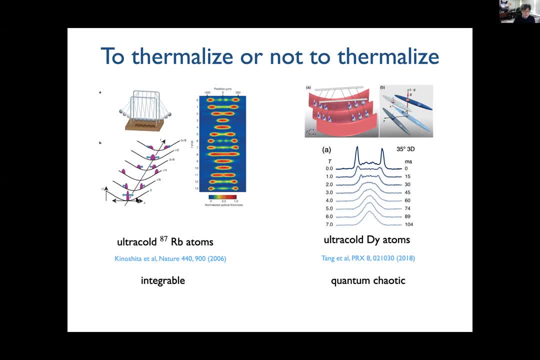 So they prepare this cold atom system in this harmonic potential and they impart some amount of positive momentum to the half of the cloud and also some amount of momentum in the opposite direction to the half of the atomic cloud. okay, So they depart in this direction, in that direction. 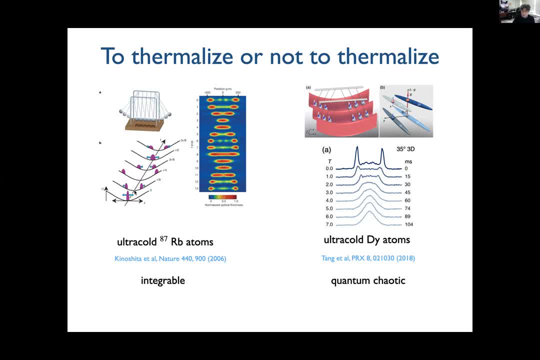 So in this initial state the system is out of equilibrium condition. but as time goes on, this atomic cloud just bounce back and forth and they do not return to this thermal equilibrium state. The equilibrium state would be some atomic cloud at the center of this harmonic potential. 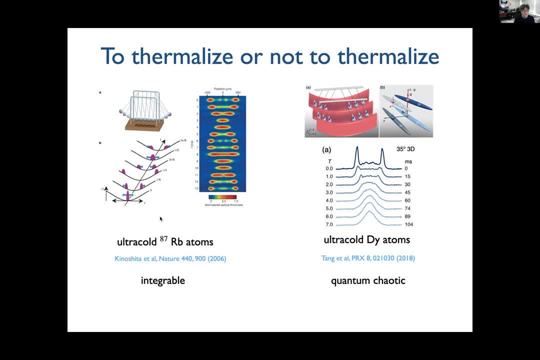 So this is some kind of an example of quantum, many-body quantum system that exhibit the non equilibrium dynamics. This is this system is called as a Newton's cradle of Newton's cradle of water-colder atoms. But if you tune the system in such a way that this atom 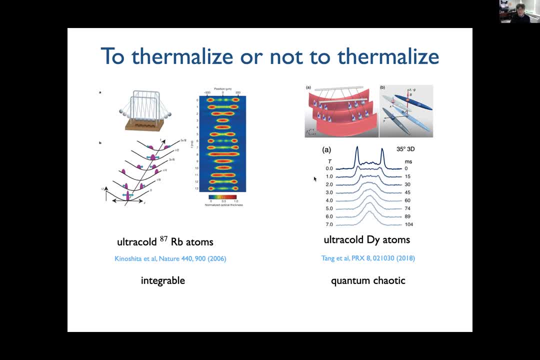 exchanges some non-trivial amount of interaction, then if you prepare the same, prepare the system in the same initial condition, but in this case the system evolves into the Boltzmann-type equilibrium distribution. So these two famous experiments show that we have now achieved such a 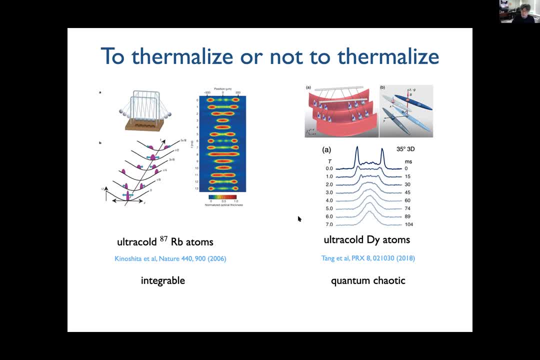 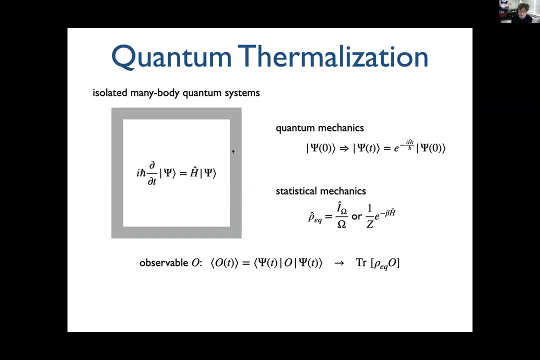 experimental technique to observe the quantum dynamics of many-body systems. And then sometimes you observe thermalization, but sometimes you do not observe thermalization. So we need to understand why or how the system is thermalized or not thermalized. So a little bit formal definition of quantum thermalization. So I have some isolated quantum system. 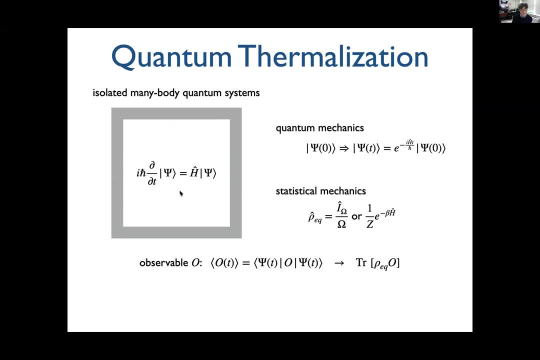 which evolves in time according to this, following this Schrodinger equation. okay, So quantum dynamics means if you prepare your system in a definite wave function, then it evolves according to this Schrodinger equation to this state. Of course, this is given by this. 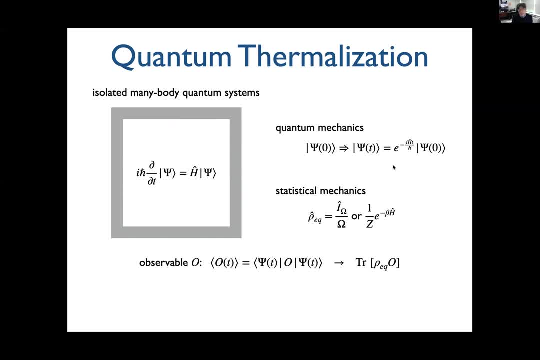 unitary time evolution- okay. On the other hand, everybody expects that if the system is non-trivial enough, then the system eventually evolves into the thermal equilibrium state, and the thermal equilibrium state is represented by this density matrix given by this micro-canonic ensemble or canonical ensemble. okay. 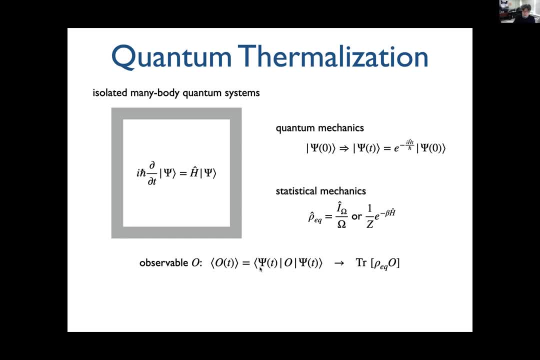 Then the question is that suppose you prepare your system in this definite quantum state represented by this wave function, psi, t. okay, Then you can measure the some, you can calculate or measure the expectation value of some local observable law. okay, Of course this should be. 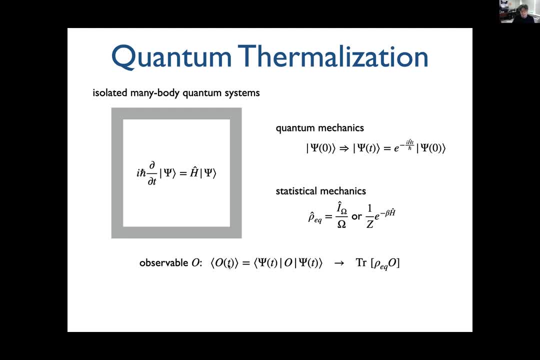 this should be a function of time. okay, Then, now you wait long enough. okay, Then the question is that whether this expectation value should approach or converge to this equilibrium, this expectation value predicted by this equilibrium, statistical mechanics ensemble average. okay, This is the. 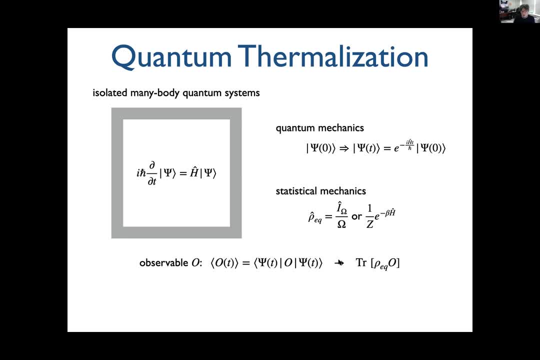 essence of this quantum thermalization. so we should check whether this happens or not. Also, you know, you know, to have this quantum thermalization, then one should this, this conversion should happen for any kind of initial state. okay, So that means 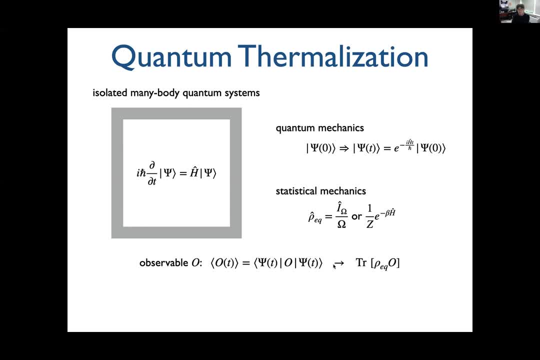 if, if your system starting from the energy eigenstate- suppose that you start your system in the energy eigenstate and then you achieve this thermalization, okay, Then that means you can achieve this kind of thermalization for arbitrary initial state, okay, So actually, 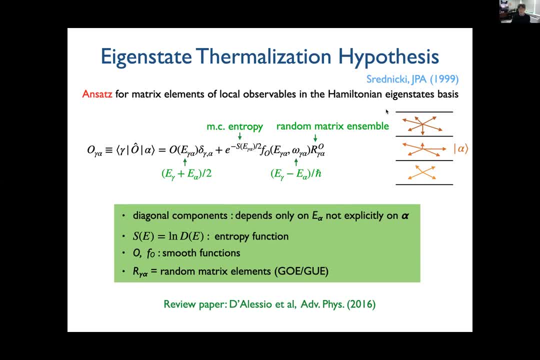 more than 20 years ago, Stravinsky proposed some kind of ansatz that guarantees the thermalization even if you start from the energy eigenstate. Okay, so this is a very this. at first sight it looks very complicated, So this is the ansatz. 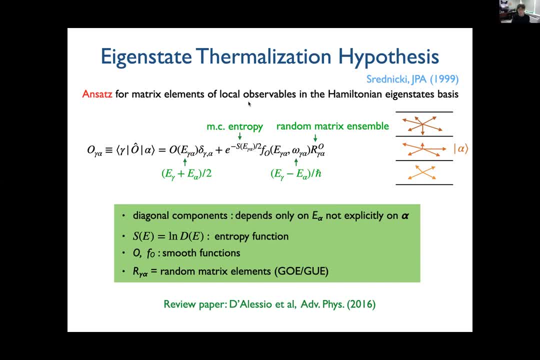 for some matrix element of local observables in the Hamiltonian eigenstate basis. okay, So if you calculate this expectation value of operator O with respect to eigenstate gamma and eigenstate alpha, then the reason that that must depends on this quantum number, gamma and alpha and also some energy eigenvalue. okay, E. 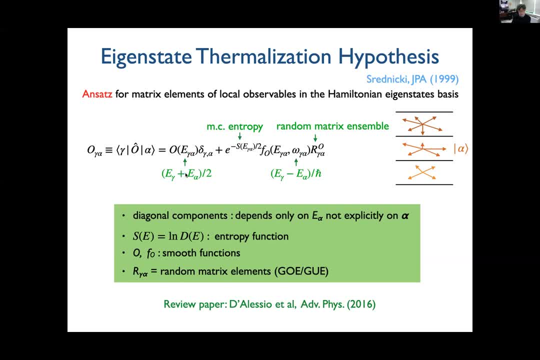 gamma. alpha is the mean value of these two energy eigenvalue and omega is the, the difference of energy eigenvalues. okay, And the so-called ETH claims that this matrix element should be written in this form in order to have achieved this quantum, so-called quantum. 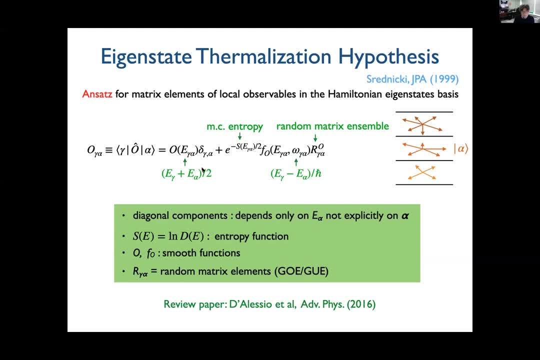 normalization. okay, So this form is very specific. For example, this is about the diagonal component. okay, So I have a chronicle data here. So this claims that the matrix element of the diagonal element should depends only on the energy parameter, not the quantum number. okay, So 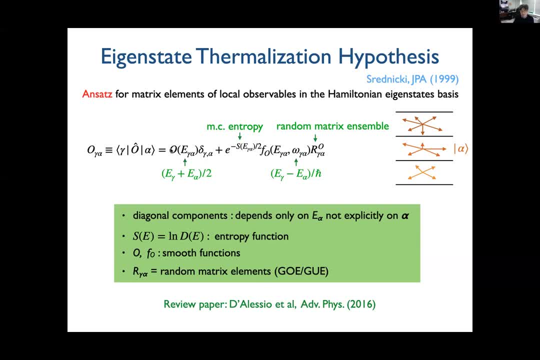 this must be given by a certain function. O, okay, There's one question. Yeah, Jay, there is a question by Arkadiy. Arkadiy, maybe you can go ahead, Yeah, so my question is like: in a previous slide you were talking about that. 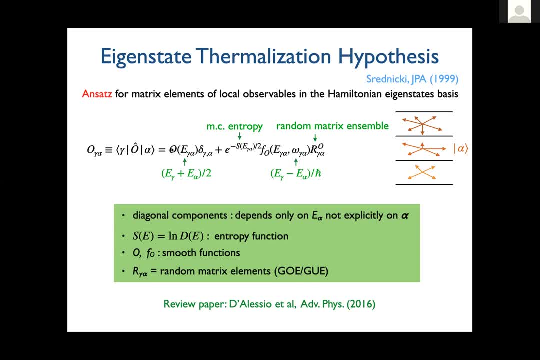 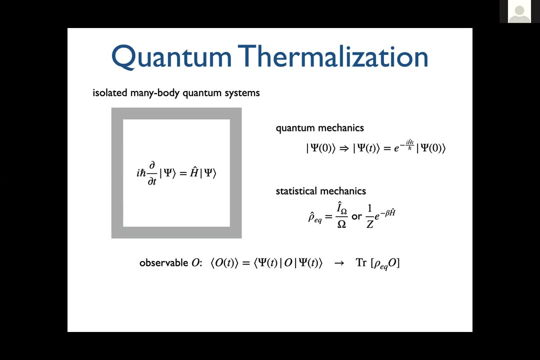 equivalence between that trace over the density matrix versus the average over the state right. Can you go back to the previous slide once again? Yeah, So wouldn't this be obeyed if, say, the rho equilibrium, the rho and the psi, the rho is like a pure state In that case won't. 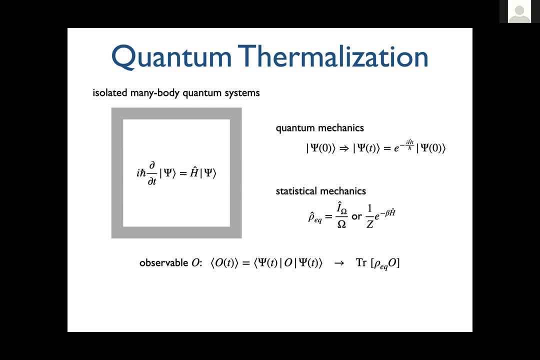 this equivalence always hold? So will that be a like thermalized state or No? no, If I understand your question correctly, this is a very specific form of denser geometric given by this micro or this. Okay, I see. 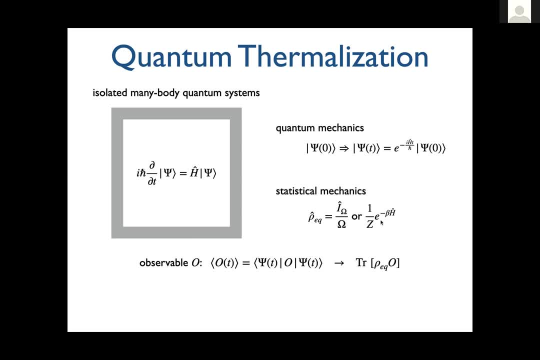 So the condition of the denser, okay, Right, So the condtion of the denser, okay, Okay, Okay, Okay, of thermalization is so it's not that both are. whenever both are equivalent, that's thermalized. 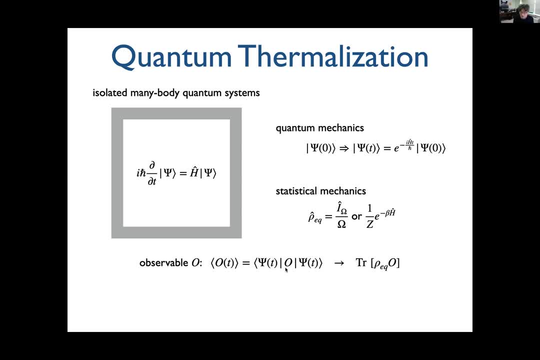 That's not the condition. Yes, yes, So this is a quantum mechanical expectation from a definite wave function And this is the expectation from the theory statistical mechanics. Okay, okay, And when they're equal, you say it's thermalized, right? 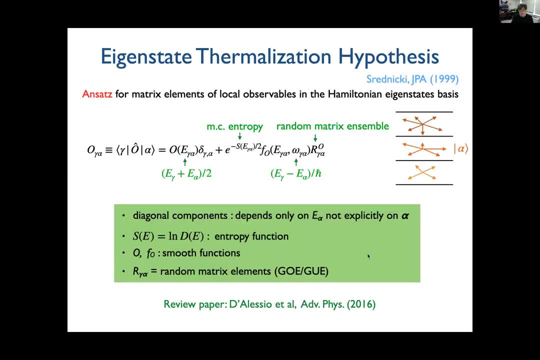 Yes, Okay. So the first part is that the diagonal component and the first important point is that the diagonal element should depends only on the energy part, not the quantum number. And this is something about the off-diagonal component, And the essence of this form is that 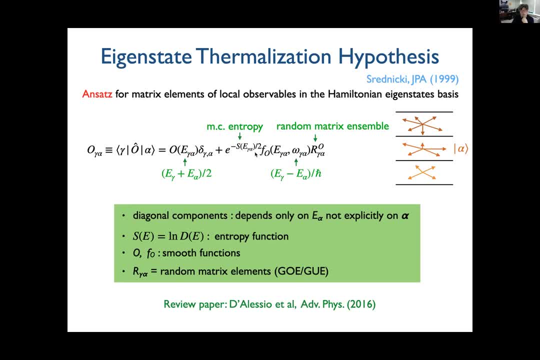 this off-diagonal component should be. the overall amplitude of this off-diagonal component is exponentially small. Okay, Why? Because it it includes this exponential entropy. This entropy is nothing but the micro slipping entropy. So this entropy is just given by this logarithm. 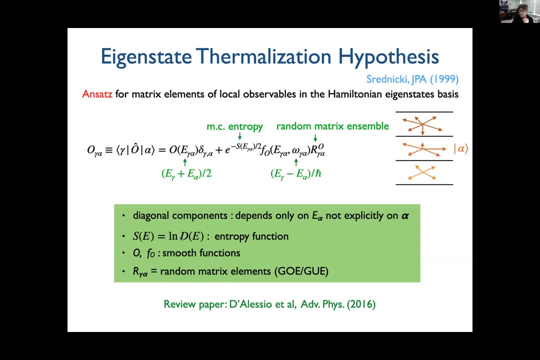 of the density of state And this is an extensive quantity in the user statistical mechanics. So this means that means this is an exponential small amplitude part Okay, And this is an amplitude and this is some operator-specific component And again this function should. 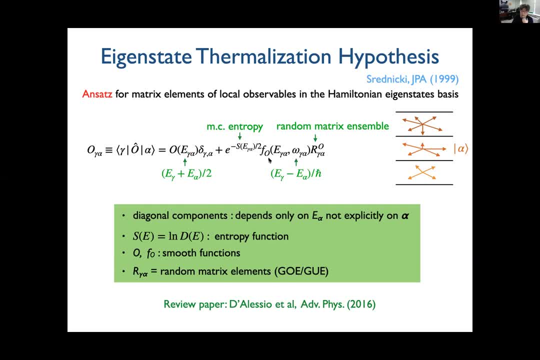 also depend only on this energy parameter, not on the quantum number itself. And, of course, if you really calculate this kind of matrix element, then you should observe some energy quantum number dependence. All such a dependence is incorporated into this additional term here, And the point is that the essence of this ETH is that this eigenstate fluctuation. 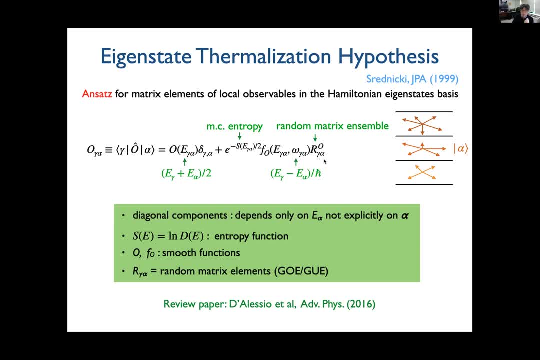 is just given by this. So actually this should obey some definite random matrix ensemble distribution, for example Gaussian or Sorbonne ensemble or Gaussian unitary ensemble, depending on the symmetry of your system. okay, So it's a very, very restrictive assumption for. 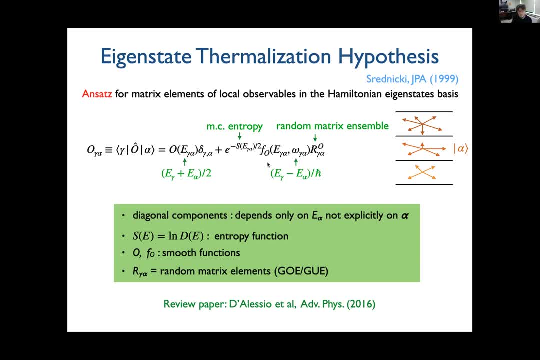 the matrix element And actually this kind of unjust is coming from the random matrix theory. So in a simple word, this unjust means that if you have, if you diagonalize your Hamiltonian- and this is the energy direction- then in each energy window you have some. 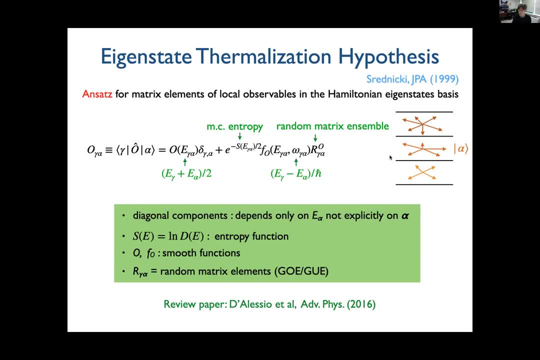 so this is some so-called micro-Kernelkahn window, and then the energy eigenstate in this window should be the same. So this is the main idea for the for this one, this unjust ETH, And so there is a very nice review paper, And so then, as I said before, this is a very, very, very very. 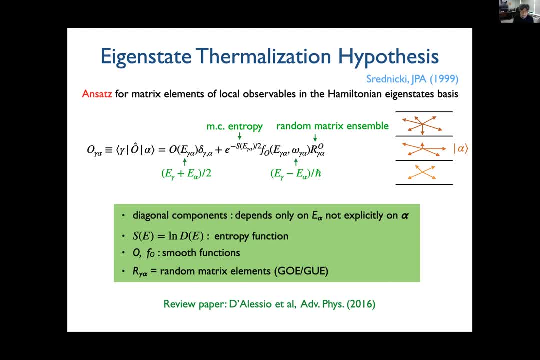 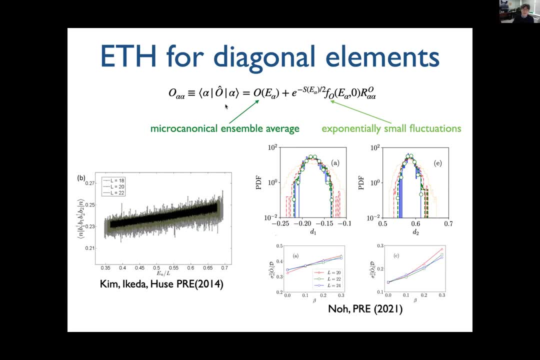 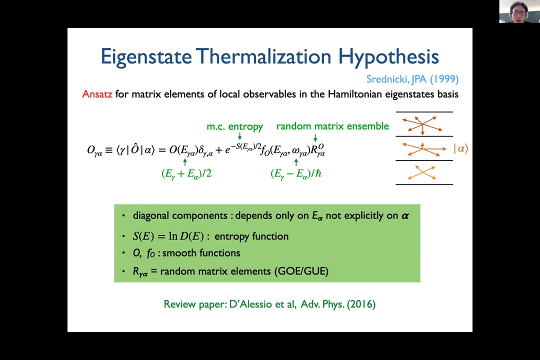 good example for us for any kind of interesting theory. Okay is a random matrix elements And maybe I missed it, but I don't understand where the randomness is coming from in this picture. So actually I have a definite Hamiltonian, So actually there is no randomness, okay. 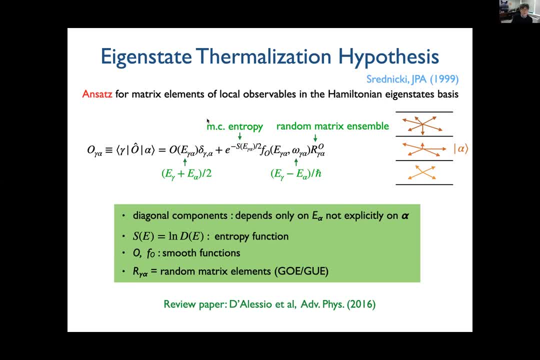 In principle okay So, but once you have some definite Hamiltonian, you can diagonalize the Hamiltonian and then you can calculate this matrix element. okay, And then you can investigate the distribution function of this matrix element. okay, You can draw this some histogram or whatever. okay. 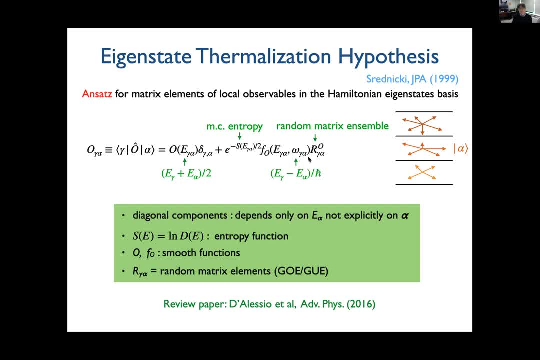 Then this claim means that if you look at some statistical property of this diagonal component, then you cannot distinguish the distribution property from that of random matrix ensemble. Oh so, So if you do, if you sum the sum of the dice, actually there is no randomness. 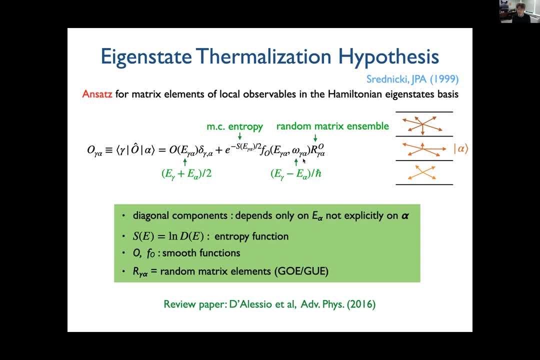 It's the solution of Newtonian dynamics, okay, But if you collect all this output of experiment, then you can compare this experimental output with this uniform distribution or whatever. okay, So this is the mean of this random matrix ensemble. Thank you. 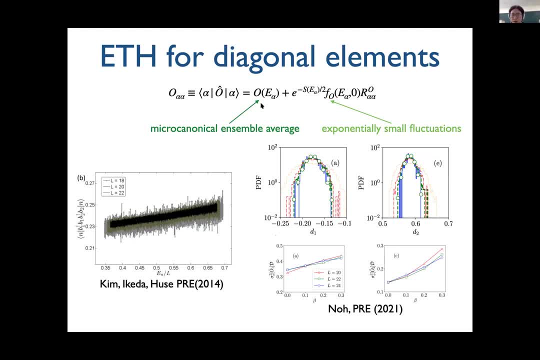 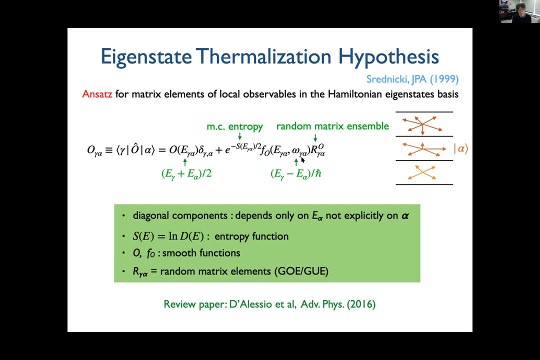 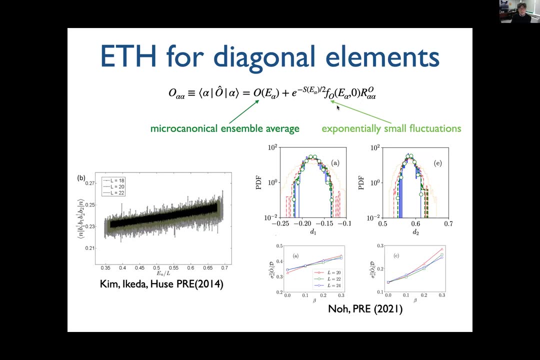 Okay, so this is the answer for the diagonal element. So this is coming from this part And, of course, there you can also have contribution from this part here. So the ETH for the diagonal matrix element means that this expectation value is given by some function of energy. 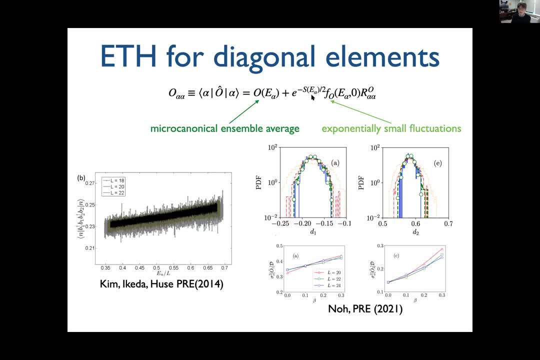 I can do that, So that's what we've got here. As I said, when you can compare these two parts, you can get the time super diesem Stayer, the latent value, with some correction terms, exponentially smaller correction terms. okay. 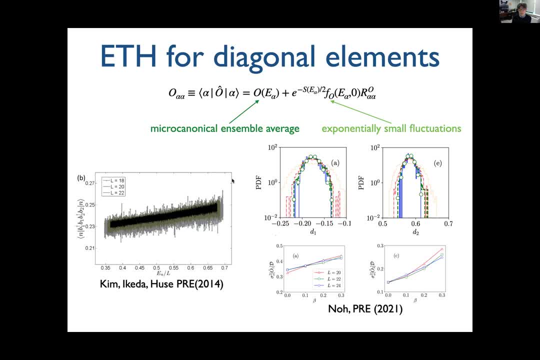 So people tested these fund using some one-dimensional spin chain or one-dimensional hardcore boson system- I mean numerically, And this shows some numerical data obtained by this group in 2014.. of this model system. but they diagonalize the Hamiltonian and then they measure the diagonal. 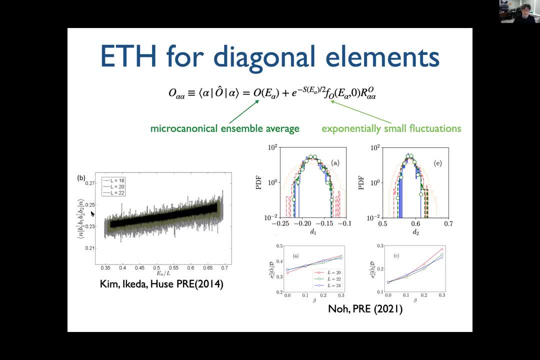 component of this specific operator, And then plot this diagonal element as a function of energy density, here by changing the system size, Then, as you can see that they tend to align along some line. This line corresponds to this function of energy. And then, in addition to that, 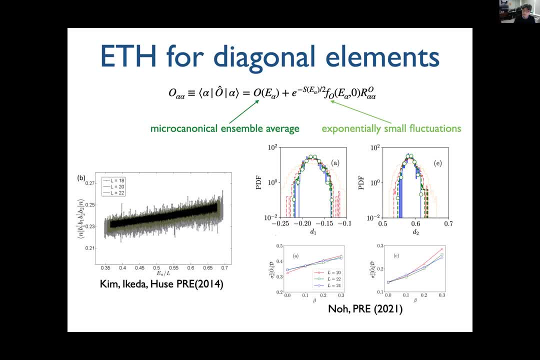 you can see some fluctuation around this line And actually this fluctuation is coming from this second part And as you increase the system size from 18 to 22,- this fluctuation, the width is just decreasing, And actually this decreasing, I mean actually this: you can check that this is an 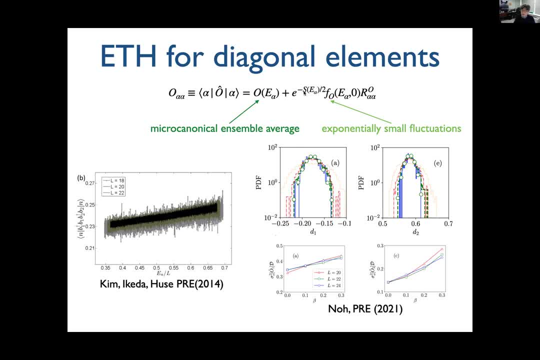 indeed, this exponential decrease according to this part. So this is some numerical demonstration of the ETH for the diagonal element, And then this is my own data. Then, now you have this, some definite your data And then you pick some numerical data within some energy window, And there are many. 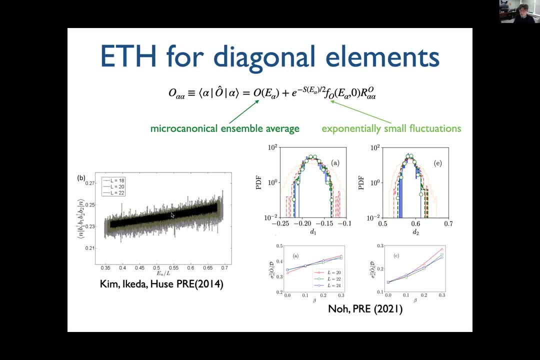 expectation values. Then you can draw the histogram And this shows the histogram. So from a small system and larger and larger system size, And then you can see that it has. it follows some this Gaussian distribution And the variance of the or standard division of this. 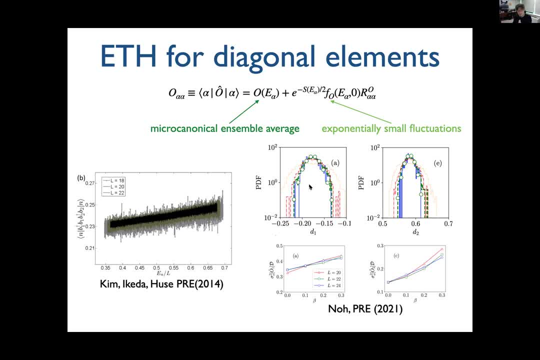 Gaussian distribution is decreasing with the system size exponentially. So there are many other. also. there are many numerical tests for this diagonal element And all the diagonal tests consistent with this ETH, as long as your system exhibit the quantum thermos. Okay, there is one question from Dominic. 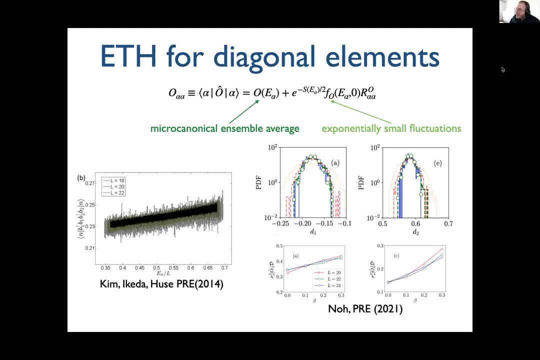 Please can you turn on your mic? Yeah, sorry, I still wonder about the x and y-axis. So what's b1?? Is that the dimension? And what's on the y-axis? Because you say it's histogram. So what is it? 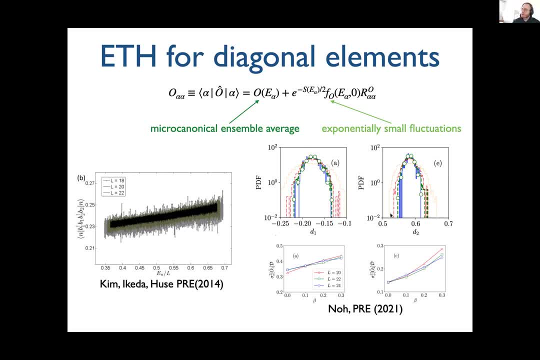 From this part or that part. Oh those, yeah, This is them, Like this here. Yeah, So d means diagonal component. d is a diagonal component of certain operator, Operator number one and operator number two. But there are many or components, right, So this is just one of them, or 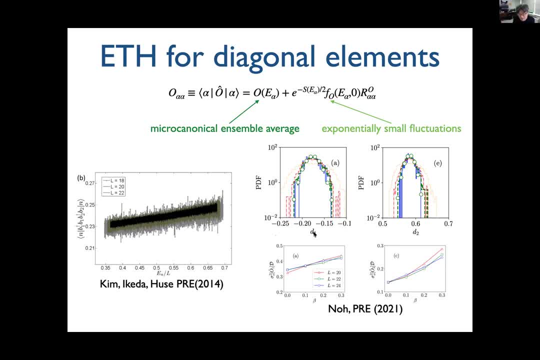 Sorry, So sorry. there are many. There are many diagonal elements, so this is just one of them. Yes, there are many, many diagonal elements. For example, within this energy window, there are many diagonal elements. So I draw the histogram of those elements. 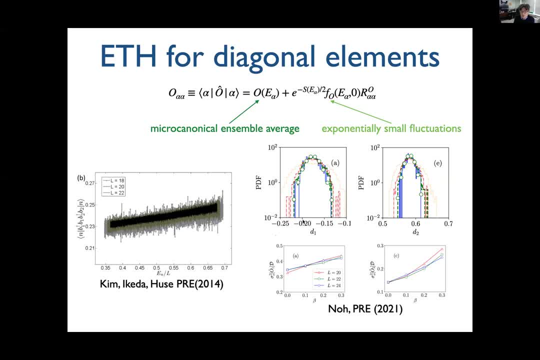 Okay, some element takes the value of, for example, minus 0.2,, some element takes the value of minus 0.15, and so on, And then I can draw this histogram. Okay, And this is data. distribution is given by the Gaussian. 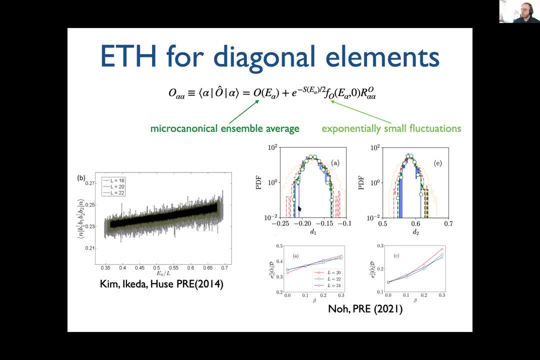 Okay, And what does it tell us? I mean how, what does it mean? What should I see in this? What does it mean? is that so? this is the answers for the off-diagonal- I mean diagonal- element ETH answers. 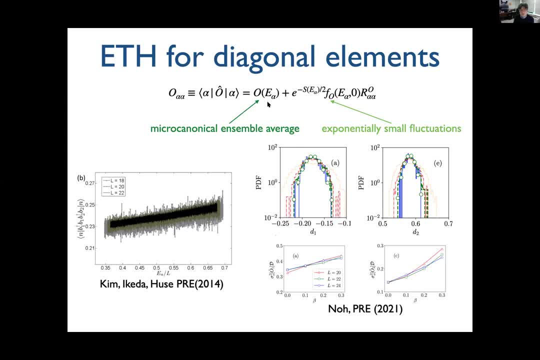 This answers means that the diagonal element depends only on the energy parameter, with some fluctuation, And this fluctuation is given by the should follow the Gaussian distribution. Ah, okay. Okay, so this is a direct test of this answers. 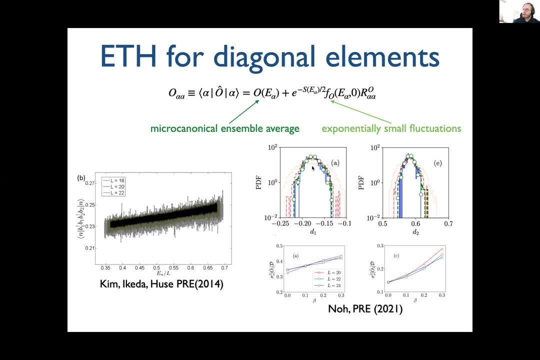 Uh-huh. So this is your data, right, But do you have the prediction data as well? or This is data, This is data, this is the prediction. The prediction means that the shape of distribution function should be Gaussian okay And the width of distribution should exponentially decrease. That's the 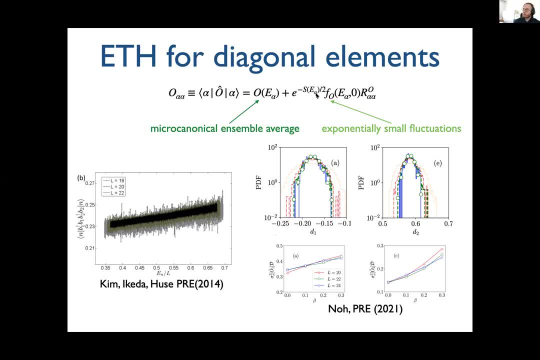 prediction of ETH. Right, but you didn't. you didn't put the curve that depends on the entropy, right? Because you don't? I don't see anything. Okay, so this is the entropy, and entropy is nothing but the density of state. okay, So, and here, the D is the density of state. okay. 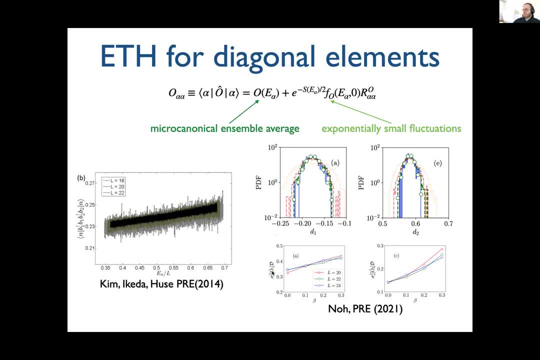 Oh, okay, So here I plot the, the variance of this distribution and and the density of state changing the system size and they, they, I mean they converge to. I mean, for example, for different system size, they have the same value means that 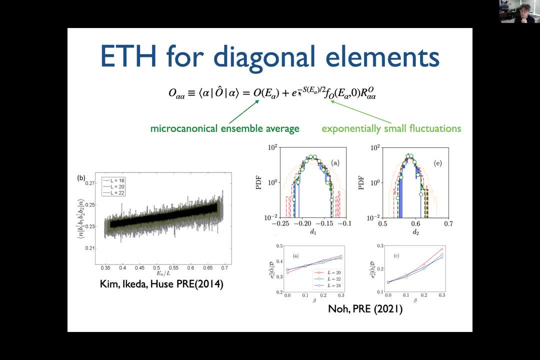 this is the direct check of this, this vector. Okay, I see, Thanks, And there is another question from Juja, So just a simple question here. So you took the entropy as a microcanonical one, and how sensitive are these results to the definition of your entropy? 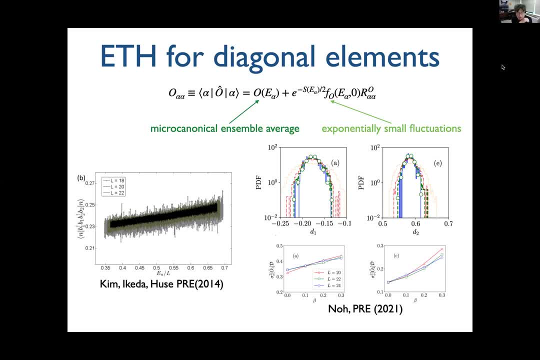 So once everything is well fitted to the microcanonical ensemble, then using this- so everything is well fitted to the microcanonical ensemble, then the system is thermalized. okay, Then, once you have a thermal system, then you can use this ensemble equivalence. 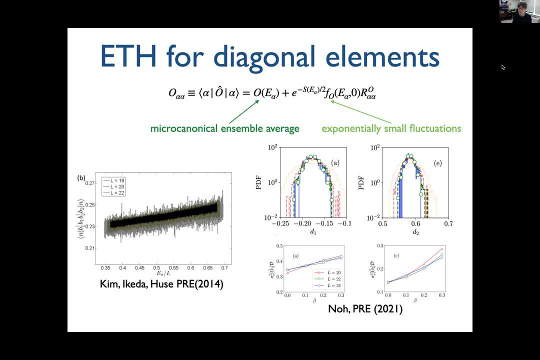 okay, Then you can translate every result from the microcanonical ensemble to the chemical ensemble. So actually, yeah, So by definition here this is the microcanonical ensemble, but if you take the Alexander transformation, then you can always transform this to the chemical ensemble. 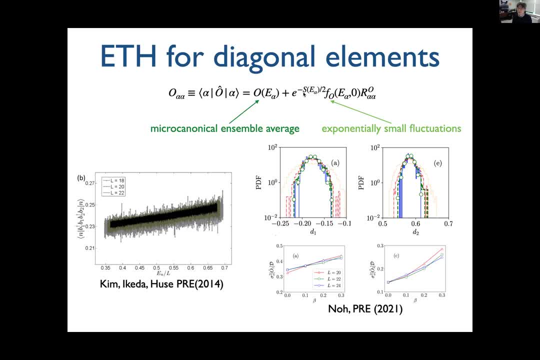 entropy as a function of temperature. So here it's good to, I mean, stick to the micro-canon, because everything is clear. I see, thank you, I thought there was another hand raised, I don't see. oh, Dario has a question. Yes, Dario, go ahead. 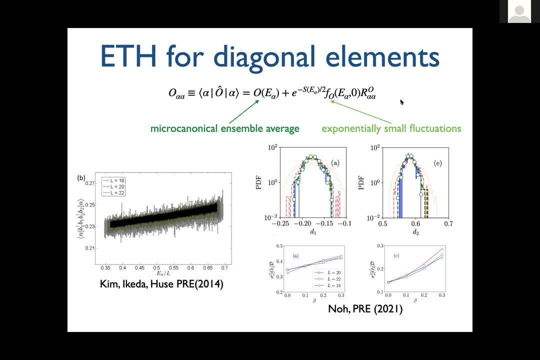 Yeah, probably related to Juzar's comment. Can we say that when we move from, let's say, micro-canonical to canonical, effectively what you are doing is a redefinition of the splitting between the exponential and the FOEI, because essentially I mean here you are splitting. 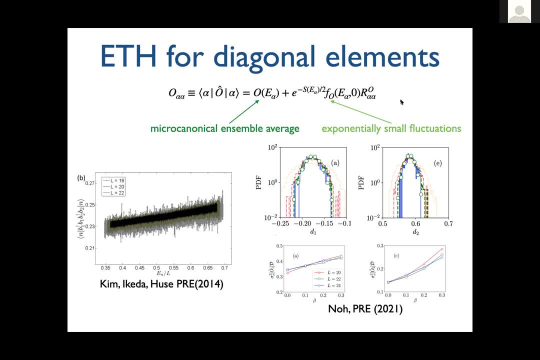 I mean you have the random matrix part which is R, alpha, alpha, O, and then you have a splitting between a function and the exponential of the entropy. If you change the definition of the entropy effectively, you are redefining what is your smooth function, Am I right? 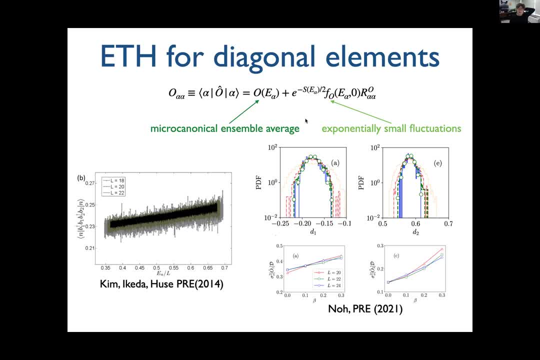 You can think in that way, but here, conceptually, we are focusing on the isolated quantum system. so I think it's better to stick to the micro-canonical example. So first of all, I mean, it's easy to take everything. 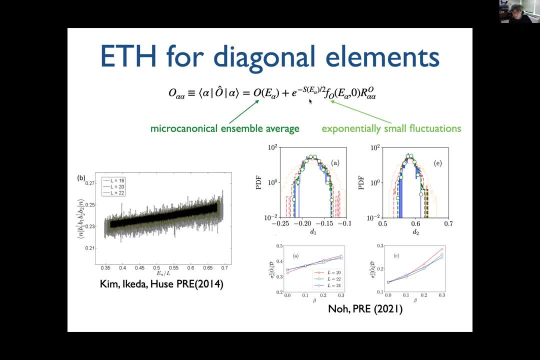 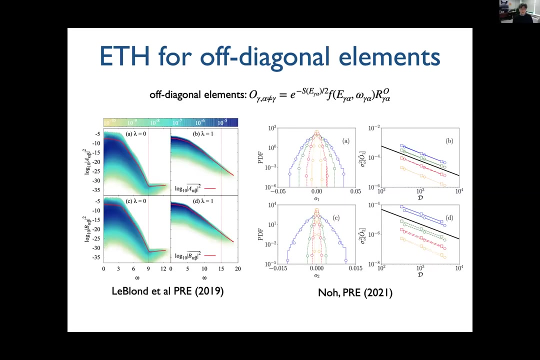 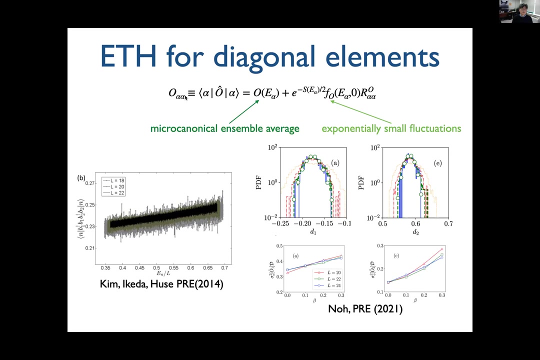 in terms of micro-canonical example. Okay, Yes, Okay, then for the moment I'll proceed and then back to this issue later. okay, during the discussion. Okay, so I showed you that the diagonal ETH and then okay, then let's move to the off-diagonal. 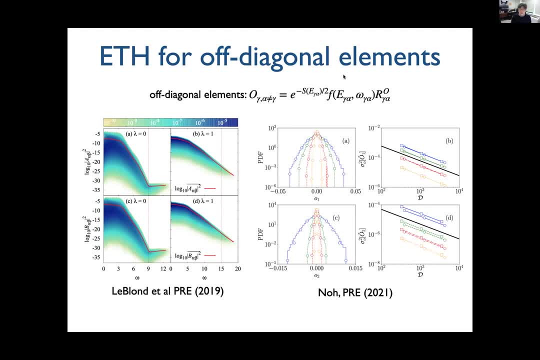 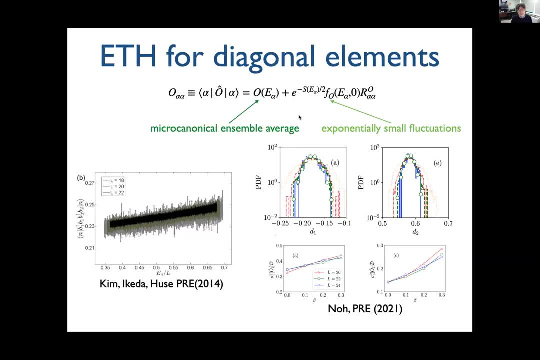 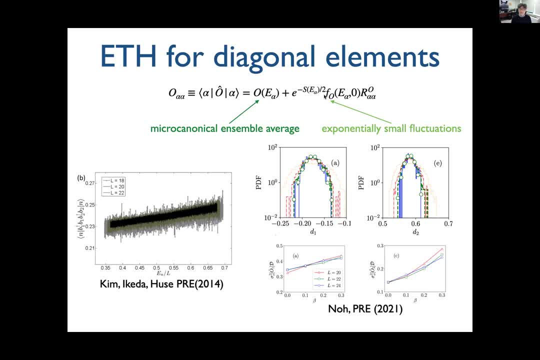 Then what does? what's the meaning of this ANZAS? Okay, So this is exponentially small, so we can ignore this part in the thermodynamic limit. Then the remaining term is not only this part and, as you can see, this only depends on the 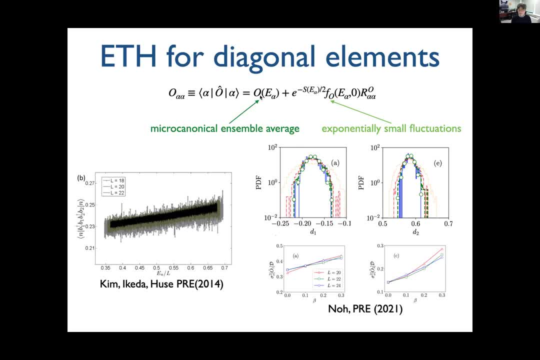 energy parameter. not on the energy parameter, Not on the energy quantum number. okay, This means that. so if you consider micro-canonical energy share, then for every energy state within this micro-canonical energy share, their expectation value is equal to each other. okay, 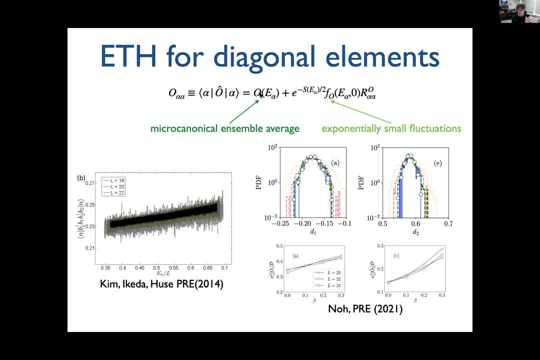 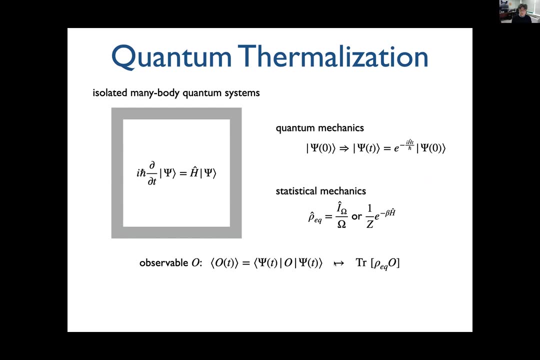 That means individual expectation value should be equal to the micro-canonical, for example, average, because every, every element should have the same value. okay, So this form guarantees the, the. the guarantees this. I mean convergence of the expectation. 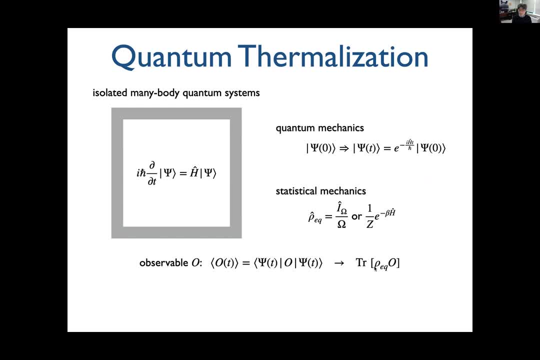 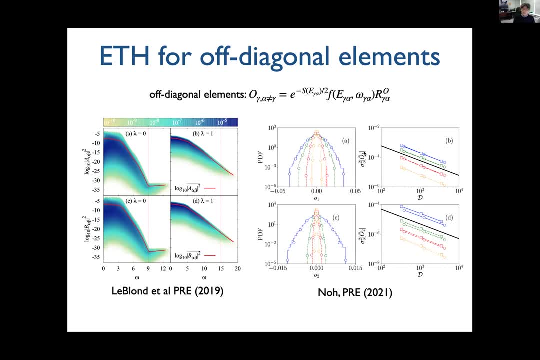 value to the micro-canonical ensemble average. okay, Okay, Then let's move to the off-diagonal element. Off-diagonal element looks like this one. I do not have this dominant diagonal component, but this. I only have this floating part. 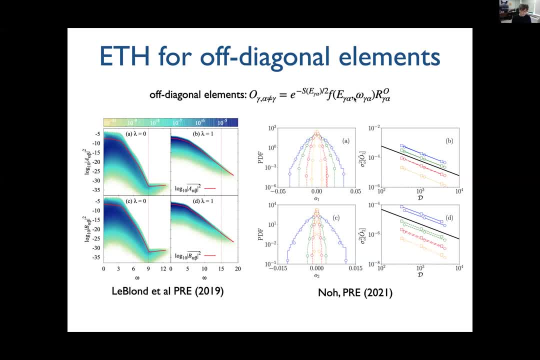 So actually this part, this form has also been tested for many years. For example, here they: they also chose some XXG chain or some spin chain or hardcore bosonic system and bring some observable Here. they represent A or B. okay. 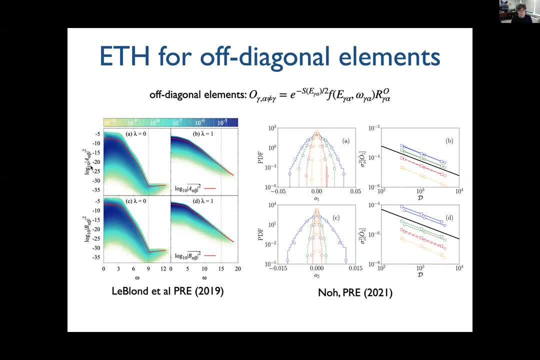 I do not show the explicit form of this operator here, but so they they measure this off-diagonal element, And so this is kind of a scatter-plat of this off-diagonal element. okay, So so off-diagonal element involves two on index, and alpha and beta. 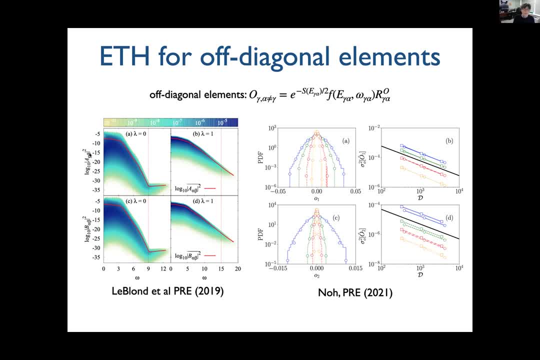 Okay, So they focus on some energy space where E-alpha plus E-beta is equal to zero, For example. okay, And then they change it this omega. Omega means the difference of intensity in the energy of the element. Okay, So it's like cool. 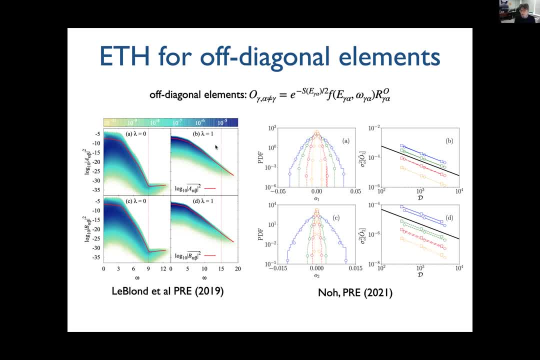 It's like, okay, Okay, difference of energy, eigenvalue, okay, And, as you can see, they are very broadly distributed and actually this broad distribution is nothing but coming from this random matrix part. okay, And you can also measure the distribution function of this matrix element. So this is. 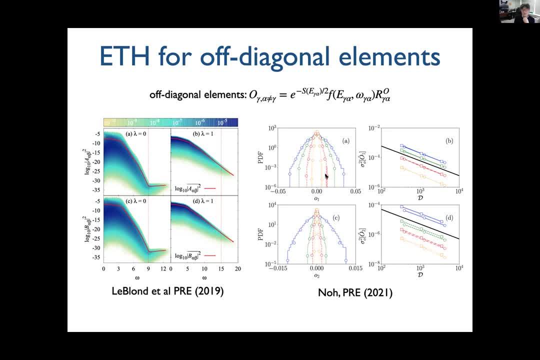 the data of mine. So I focus on some part of energy space and then calculate all the off-diagonal component and then measure the histogram, construct a histogram of off-diagonal element from small system size to larger system size. okay, As you can see actually, 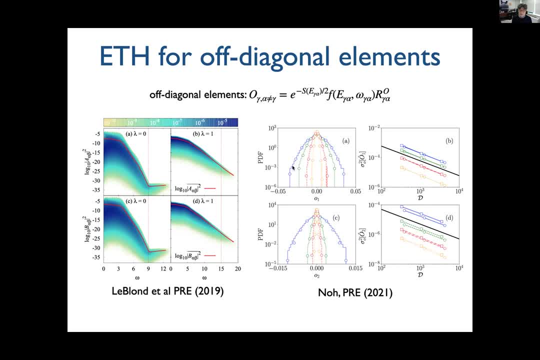 this line is the numerical data and this symbol is the Gaussian fitting, So we can see this is a perfect match here. okay, So this numerical test confirmed this Gaussian nature of this fluctuating part, and also you can measure this standard deviation or variance, and this standard deviation is also, I mean, the variance of this. 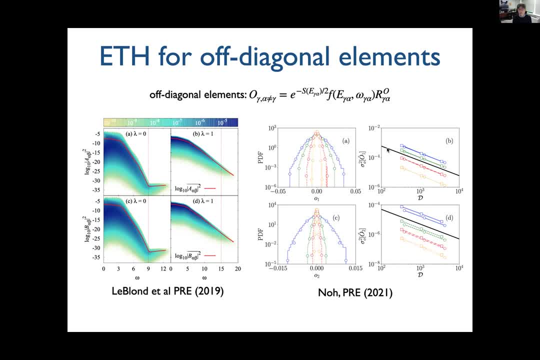 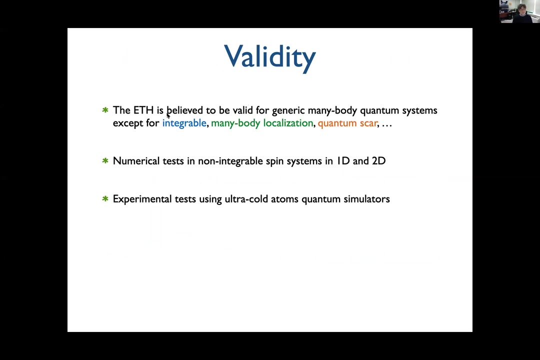 distribution. it's shown to be inversely proportional to the density of state. I mean that. So this conforms, this exponential part, Okay, And so this is kind of a numerical study to confirm the ETH, And so a brief summary. So now many people believe that ETH is valid. for some. 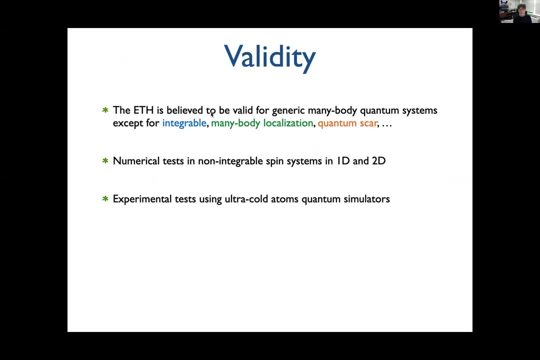 general many body quantum system which guarantees the quantum thermalization. This is kind of a main mechanism for the quantum thermalization of isolated quantum system. But of course there are many exceptional cases, For example integral system. Integral system is something similar to. 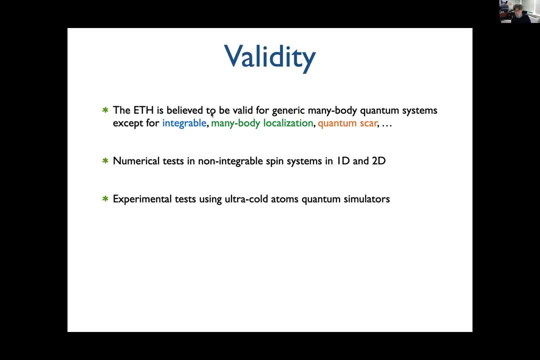 the harmonics related system, The first experimental system I showed you. Okay, That system do not thermalize. Okay, If the dynamics is too simple. for example, if your system is non-interactive, then there is a problem. So the system is not thermalized. Okay, If the dynamics is too simple. 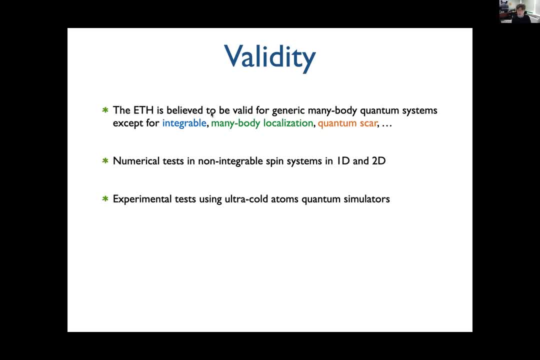 there is no reason to expect thermalization when it is isolated. Okay, Even if you have some amount of interaction. still, system can be integral. Integral means you have macroscopic amount of conservation law. This conservation law prevents your system from approaching thermal equilibrium state. Okay, So these are the exceptional case. And if your system 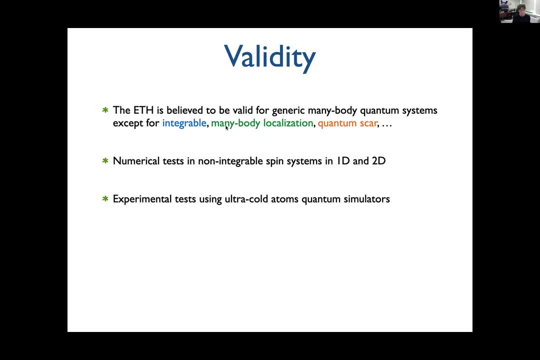 have strong enough disorder, then your system may fall into the localized phase And this localization prevent this thermalization too. And there are some exceptional cases that do not belong to integrable or many body localization scenario, But still there are some exceptional system. Okay. 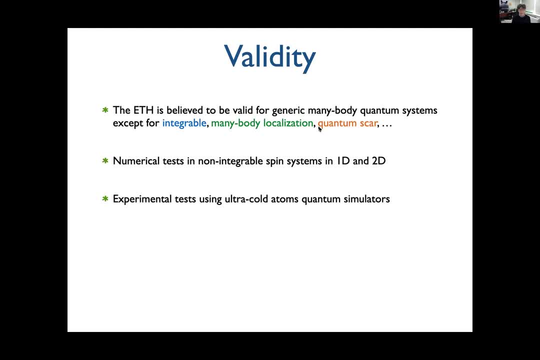 Which are known to violate this ETH. That does not follow the ETH prediction. Okay, And these are tested in many, many different numerical systems, And nowadays this prediction is being tested experimentally using the ultra cold atom systems, Using quantum simulator setups. Okay, So 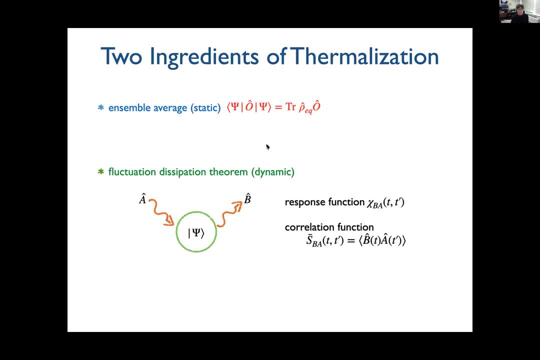 from this ETH, you can understand why you- I mean why this quantum mechanical expectation value is equal to the micro-cannot ensemble average. But this is just only a single aspect of thermal equilibrium. I call this just a static aspect of thermal equilibrium. Okay, But if you say something, 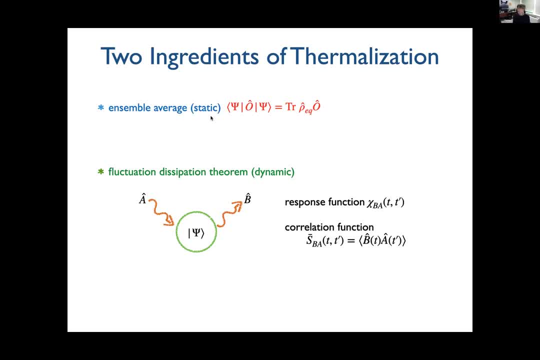 about the thermal equilibrium, then we should have another ingredient. I mean the thermal equilibrium, Okay, Okay, Okay, dynamic gradient: this is the fluctuation dissipation theorem. In the classical language. we can say that: some detailed balance or something like that. The fluctuation dissipation theorem. 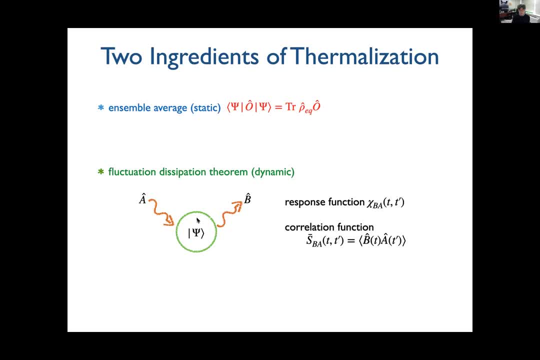 means that suppose you have a quantum mechanical system and then if you apply some perturbation, then you may have some response in the quantity of some quantity B- I mean some quantity represented by another operator B- And this response is usually described by this linear response function. 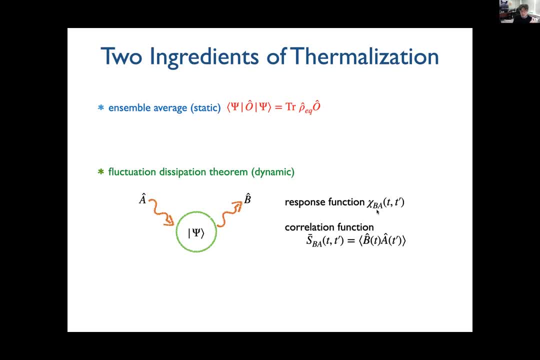 And this f is kind of a formal relationship between this response function and the correlation function. Okay, Two time correlation function And, as you can see that this is a two-time property, So this f is related to the off-diagonal f element of the matrix observable. okay, So this is from the diagonal element, but this is from the. 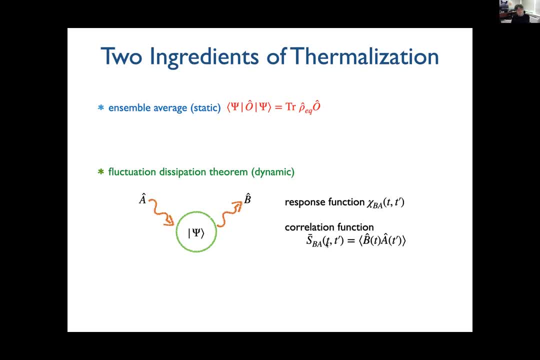 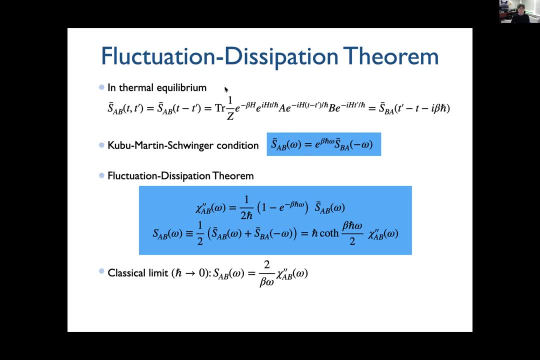 off-diagonal element. So actually. so this is the formal setup for the FTT. So suppose, if your system is in the true thermal equilibrium described by this Boltzmann distribution- okay, Gibbs distribution- then you can have some formal expression for this correlation function. But 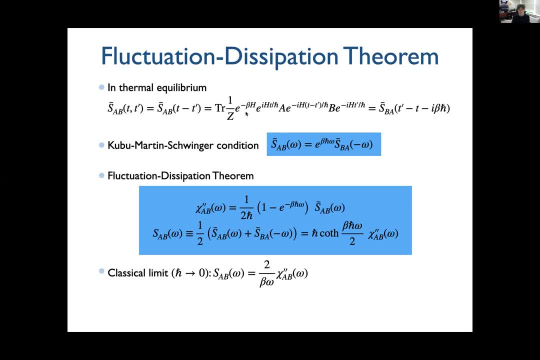 because of some similarity of this time evolution function and this Gibbs distribution, this correlation function S can be related to the another correlation function S. okay, With some imaginary time, And if you perform the Fourier transformation, then this relation is translated into the spectral. 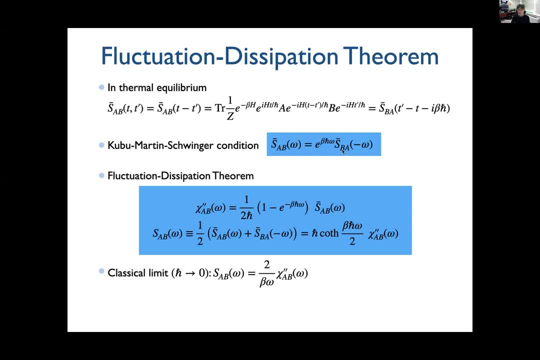 function of S and S, And S of omega is equal to the S of minus omega, with some extra factor. okay, So this kind of symmetry relation is imposed by this Gibbs distribution And this symmetry relation is called Kubas-Martin-Schwienger condition. Sorry, there's a keeper here. I'm terribly sorry for. 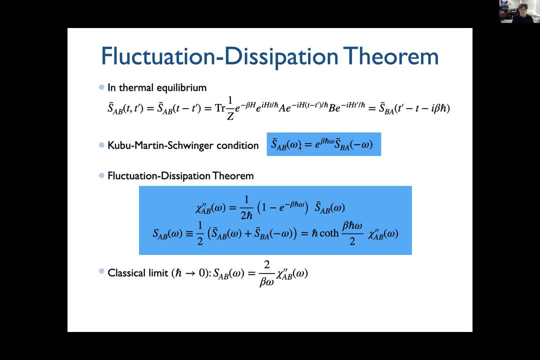 that, okay. AndNOW then, what about the, the response function? Actually, if you apply the linear response theory, then you can have some kind of formal representation of this response function. okay, So that's acription, Okay, Heroic distribution, okay, is密 sportable. 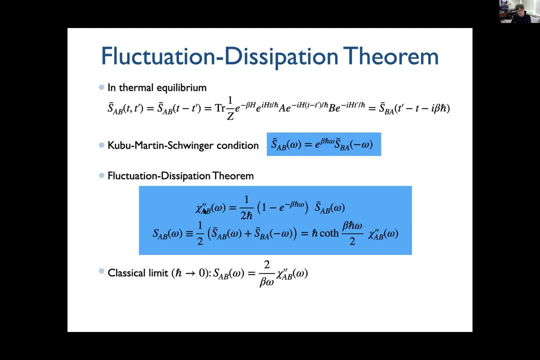 So, using this linear response theory, then you can establish this, the formal relation between response function and this correlation function. and also, if you apply this equilibrium condition, then you end up with this famous fluctuation dissipation theory for quantum system. So it's easy to work in this symmetrized form. 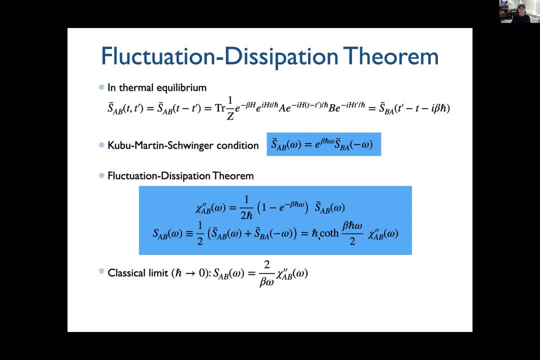 of correlation function, then this correlation function is proportional to the response function with some factor here. It looks very strange, but if you take Planck, constant h bar goes to zero limit, then you recover this some familiar form. This is nothing but the classical version of the fluctuation dissipation theory. 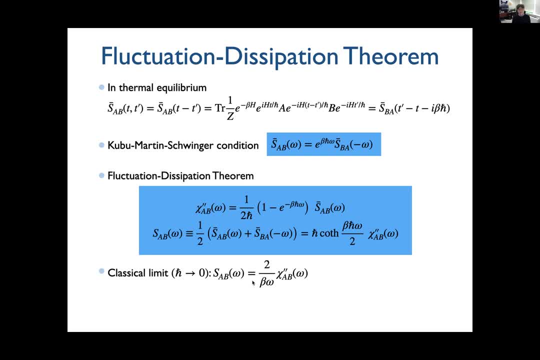 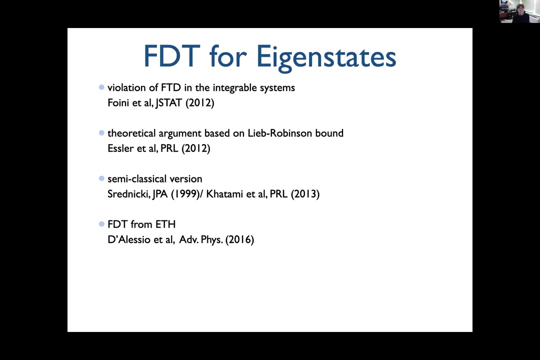 and if you take omega goes to zero limit, then you end up with some familiar FDT. for the classical system, The susceptibility is just given by the fluctuations. Okay, so actually all this, this fluctuation dissipation theorem, is based on this Kubo-Martin-Schwinger condition. So now then? 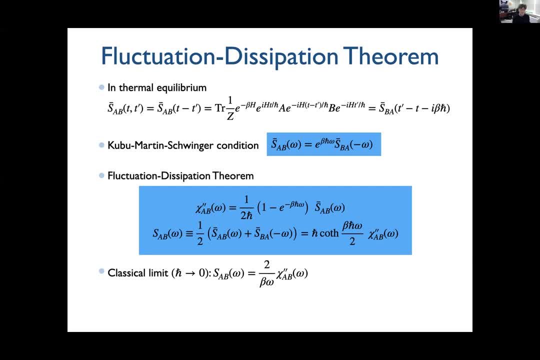 let's ask the question whether the isolated quantum system- can I mean- really obey this fluctuation dissipation theory. Okay, so there's a question. Yeah, Dominic has a question. Dominic, go ahead. Yeah, so could you, could you say what does this mean, like in physical terms? because I can see. 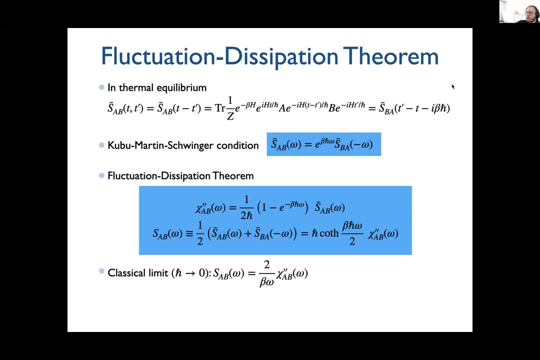 some math, but I have no clue. what does it mean? what could I imagine behind that? The fluctuation, dissipation theorem? So you mean this, the meaning of FDT, FDT? well, what are these terms there? What do they mean physically? That's what I wonder. 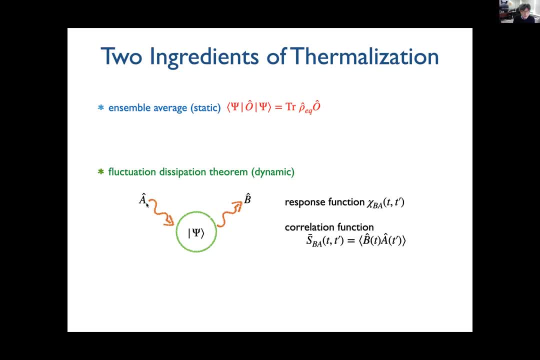 Well, in FDT it means that if you apply some perturbation, then you expect some response from the system. Okay, then that response is represented with this response function. Okay So, and then the FDT is a formal relationship between this response function and the correlation. 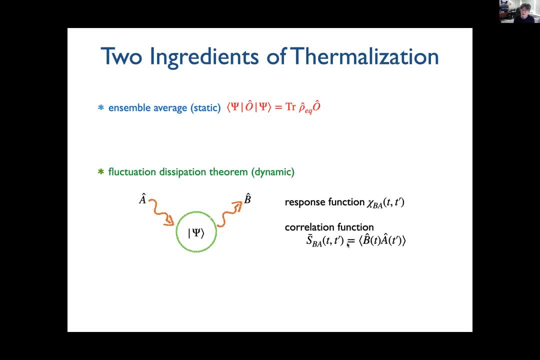 function. Okay, So actually this: these, these are these two repetitions at Again. you understand. the value is then și. these two are some kind of independent quantity. Response is in your part of your system, and what is the output of this perturbation? That's the response function, But correlation function is: 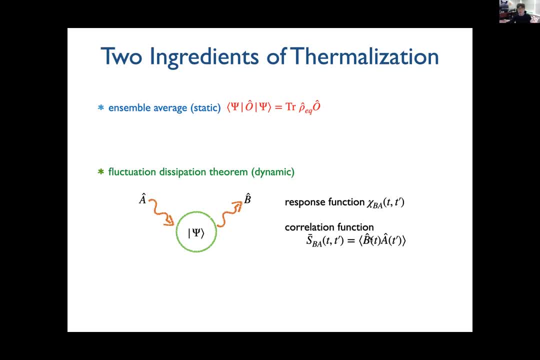 just if you take, if you give me any two quantity and then I just can compare, calculate the correlation function, okay, Then FDT means that the response is somehow proportional to some combination of these correlation functions. That's the essence of the FDT and in the classical, 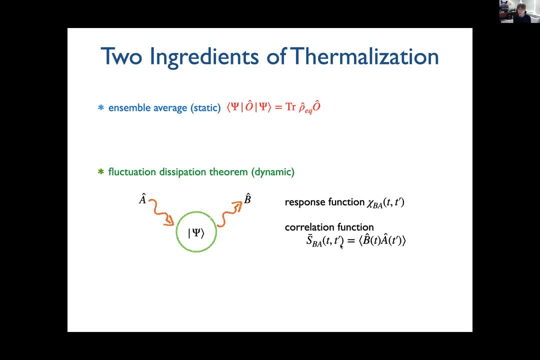 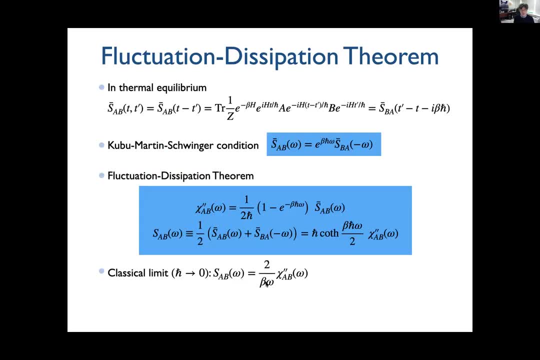 system. if your dynamics obey the detailed balance, then this, I mean we have some kind of magical, this kind of proportionality of this correlation and response function. Okay, There's a direct consequence of detailed balance in classical system and for quantum systems. 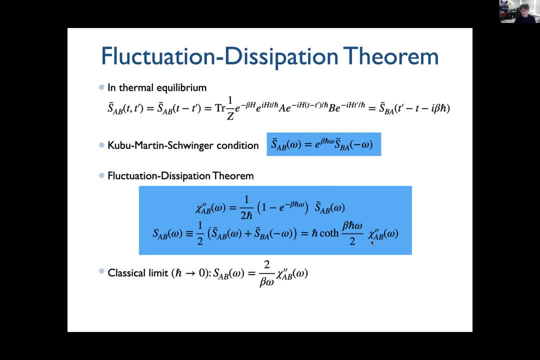 the relation looks a little bit complicated, but the essential meaning is the same: that the correlation function and the response is proportional. So if you have some very highly correlated system, then it has some sensitivity, more sensitive to the perturbation. That's the. 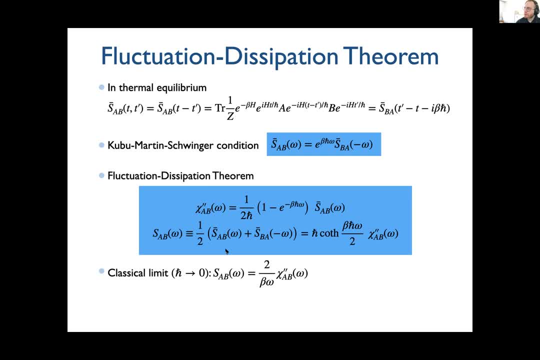 message of FDT. And this double dash, that's the second derivative. No, it's kind of the notation. This is double. that means the imaginary part of some generalized response function. but just forget it, Forget about it. Just the response function, All right, thanks. 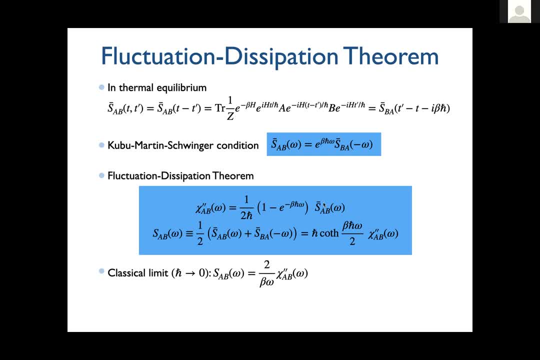 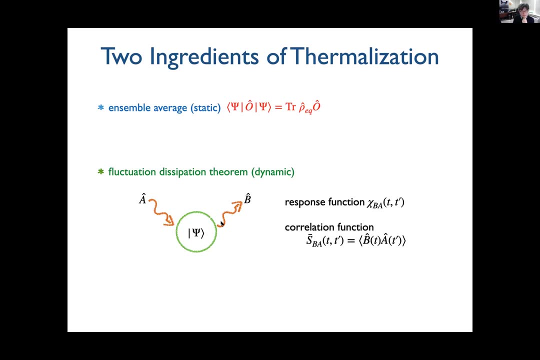 Just to mention, you have roughly 15 minutes to wrap up the talk, So I have a quick question. So how do you define the response function? Response function: okay, so in the unperturbed system you have a time. evolution of expectation of p- okay, And then, if you apply, 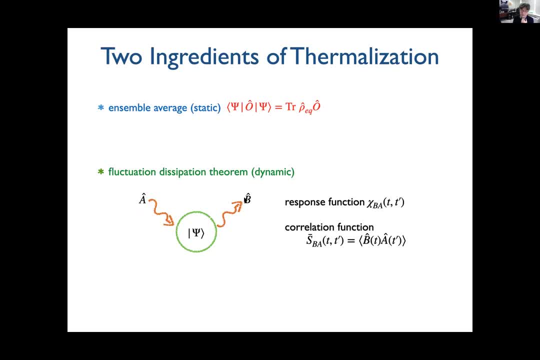 the perturbation of a. then you have some modified time evolution of b. okay, Then the response function is defined as: the difference of the response in b, The change of b with respect to this a, The functional derivative of b with respect to a. Okay, because I always find it a bit confusing that. 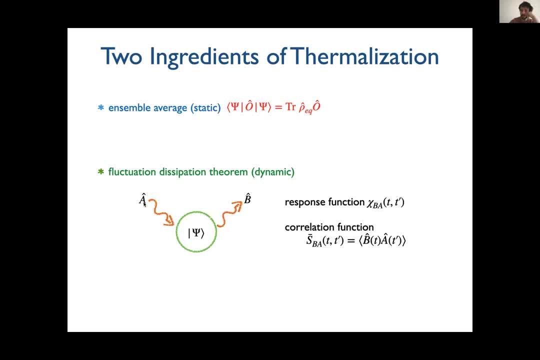 because you call it kind of fluctuations so. but oh yeah, this difference of averages, so I always Yeah. So in the classical sense sometimes we call it dissipation and sometimes we call it fluctuation. I think it depends on the context. 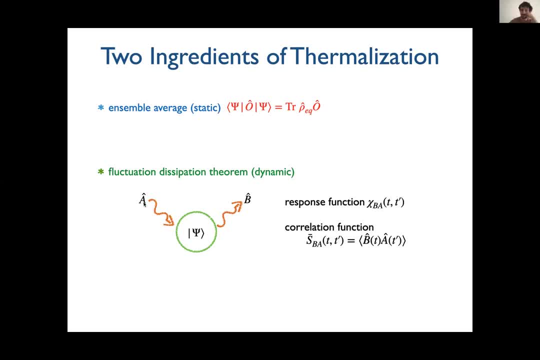 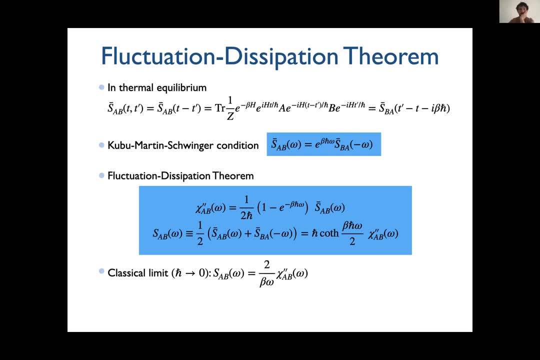 Okay, So in this context the response is correct. Okay, okay. And Dario, Yeah, somehow related. I mean, here the expectation values are taken over the thermal state. here, Okay, yeah, here you are taking the expectation value over the thermal state. 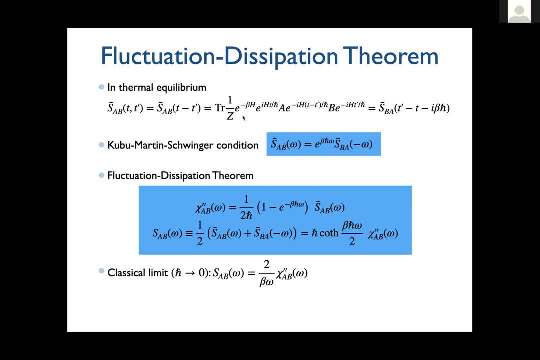 Yes, yes, But so you are already assuming that ETH holds and so thermal, let's say, behaves like a thermal state, Okay, so this is the review of fluctuation in this case, Okay. Okay, If you are already in the thermal state, then it automatically guarantees this FTT. 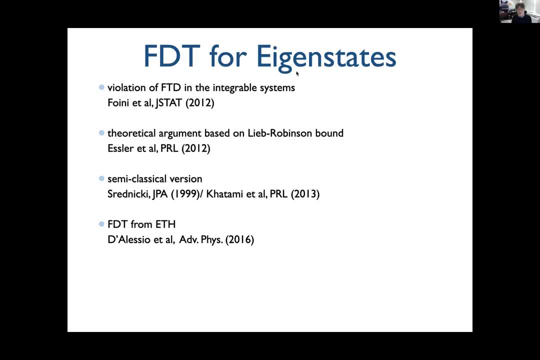 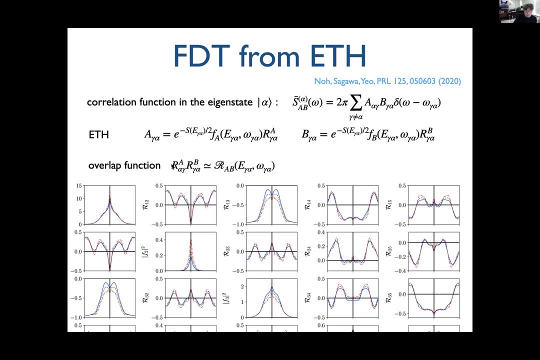 Okay, Our question is that if you start from the energy eigenstate, then still we have the FTT or not? that's the I see. Okay, got it. Sure, there are some previous work. I just skipped this, and okay, then now I am in. 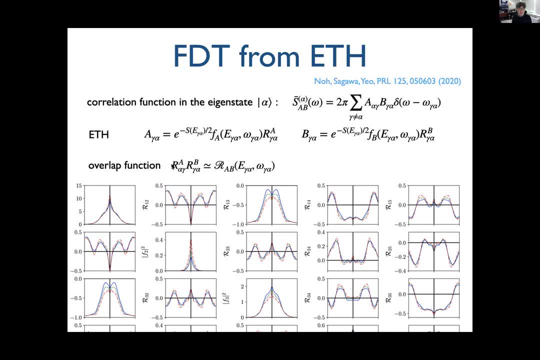 the energy eigenstate, okay, and then I assume the ETH. then can I expect the ETH and the FTT out of this ETH? that's the main question. So this is the formal expression. Okay, So this is the formal expression for the structural function, I mean the correlation. 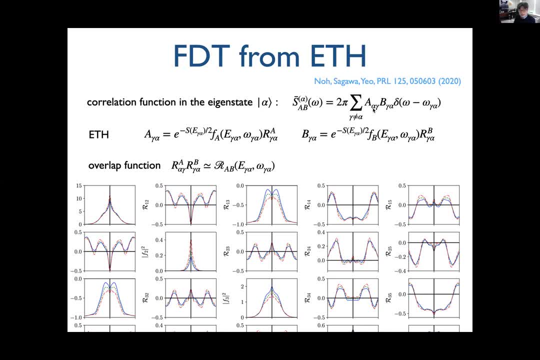 function in the omega space. okay, and, as you can see, it involves this off-diagonal component. Okay, Then, the strategy is to take this ETH ansatz into this form. okay then, okay, so there are some figures, but I just skipped this. 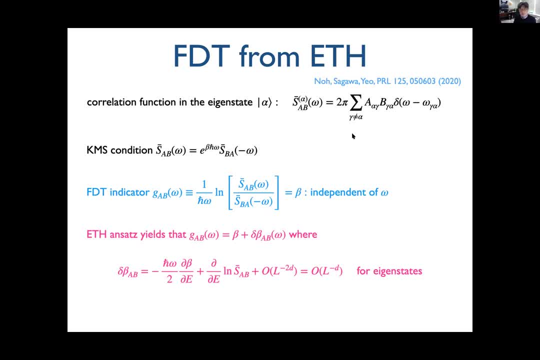 Then we should answer to this: So the expression using the ETH does it satisfy this Kubo-Martin-Schubinger condition or not? Okay, So this is: this is for the definite energy eigenstate, not not the average over the. 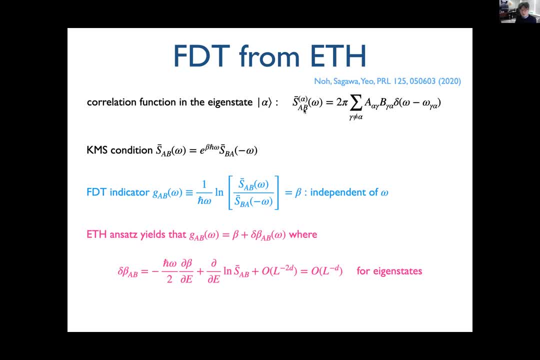 canonical ensemble level: canonical ensemble. okay, So we should check this. okay, Then, how to check this one? This check this will help. Okay, So the correlation can be checked using some indicator function. I call this indicator function GAB. 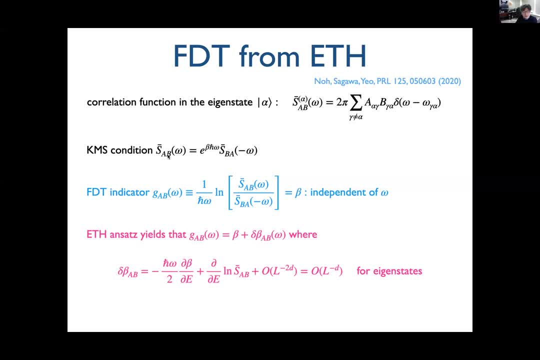 You take the ratio of these two correlation functions and take the logarithm and divide this quantity with h by omega. Okay, Then if, if your system satisfies this ETH FDT, then this quantity should be independent of omega. It should, it should be some constant. 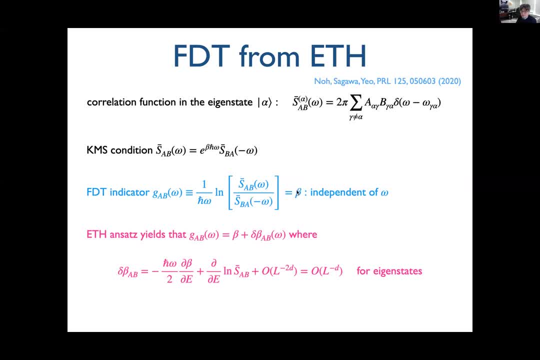 And also this constant should be independent of omega. Okay, equal to the inverse temperature. So my strategy is that, using the ETH, I will evaluate this expression and then I will construct this indicator function and then investigate whether this is convert to some constant value. I mean inverse temperature. 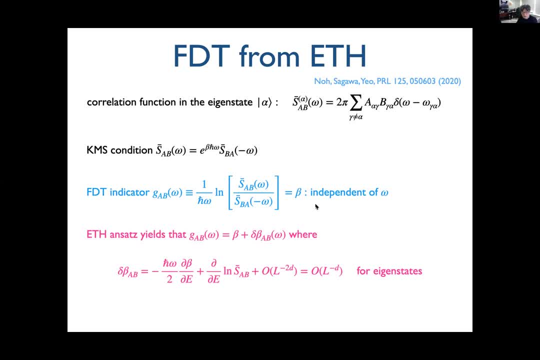 Okay, so actually there are many, some long algebra, but I just skip all this algebra and I just show you my main result. Okay, by assuming ETH, I obtain this result. this indicator function- Indicator function- is equal to some constant. Basically, this is the inverse temperature. 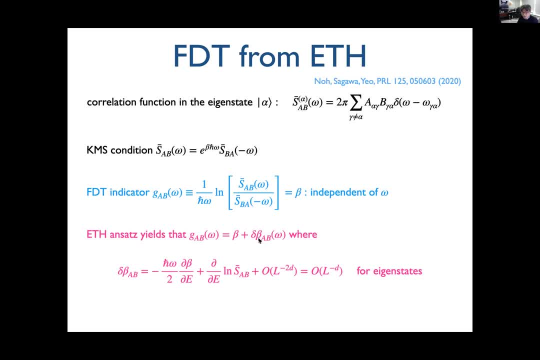 plus some correction term. This correction term means that illustrator does not obey the FDT. But this is the expression for the correction term. But, as you can see here, this correction term is the derivative with respect to some macroscopic quantity, of some intensive quantity. That means this correction term is: 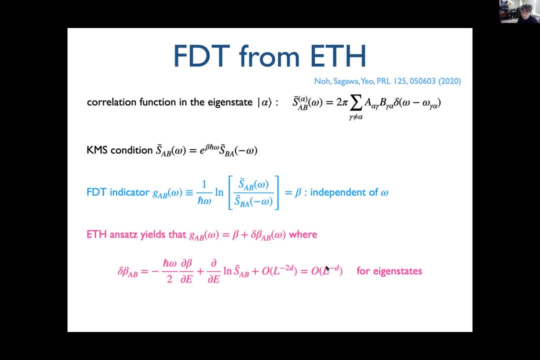 proportional to, inversely proportional to the system size. Okay, so in that sense this correction term is just a finite size correction. so in the thermodynamic limit it should vanish. That means in the thermodynamic limit we expect the FDT even in the energy. 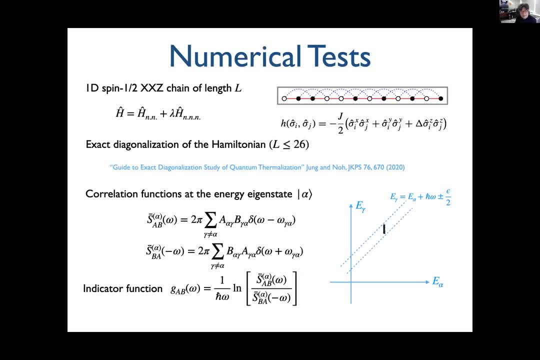 eigenstate. So I check this finite size correction form with explicitly with this spin half x-axis chain. okay, PMF-XXC chain is a one-dimensional system and I'm considering this kind of XXC interaction. So delta is an isotropic parameter of the system. 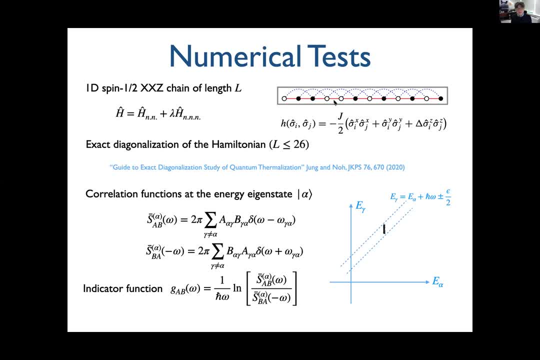 And I can think this nearest neighbor interaction, okay, This is represented by here. and then I can also add next nearest neighbor interaction, here with amplitude lambda. And it is known that without this next nearest neighbor interaction, the nearest neighbor interaction Hamiltonian is. 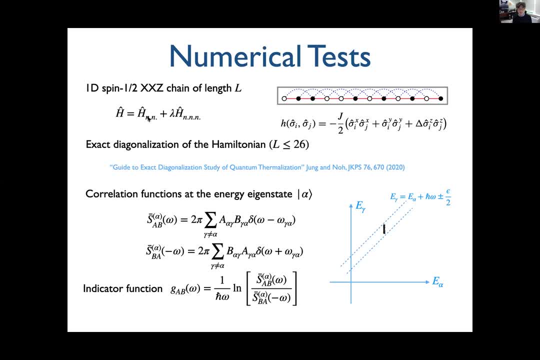 beta and that's solvable. okay, So this does not obey the ETH and this system do not thermalize. But if you introduce this lambda, then this system is known to thermalize. okay, So from this Hamiltonian I diagonalize the Hamiltonian and I construct a matrix element of various observable. 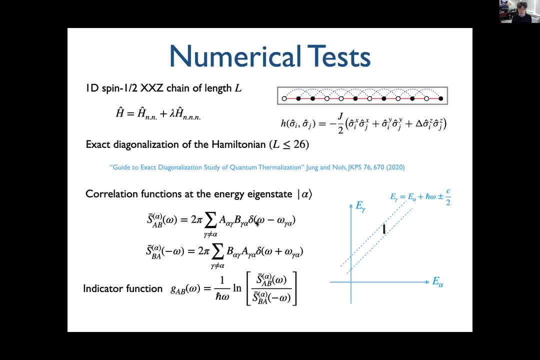 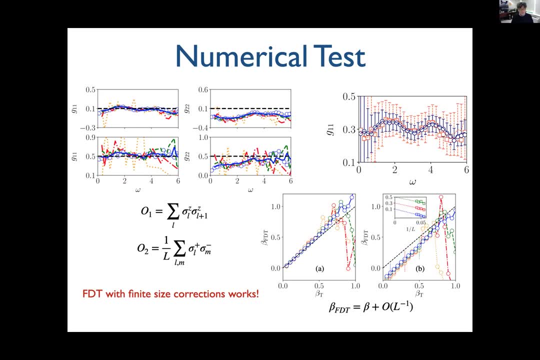 and then evaluate this correlation function and also this indicator function. okay, So this is a numerical data of the indicator function. okay, So this line is the numerical data and, as you can see, they depends on omega. okay, You can see some, some up and down behavior. 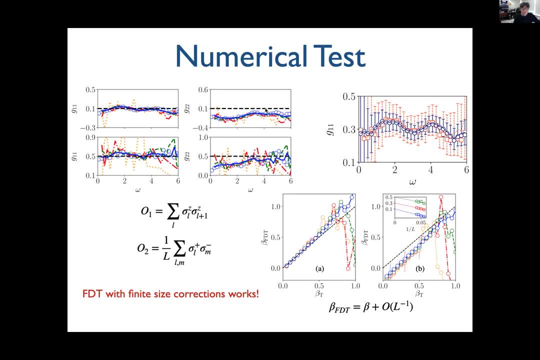 And this dashed line is the expectation from the thermalization scenario. okay, So it is deviated from this, this value, and also there is some fluctuation. But what we found is that actually, this deviation and this fluctuation is really, it's perfectly described by 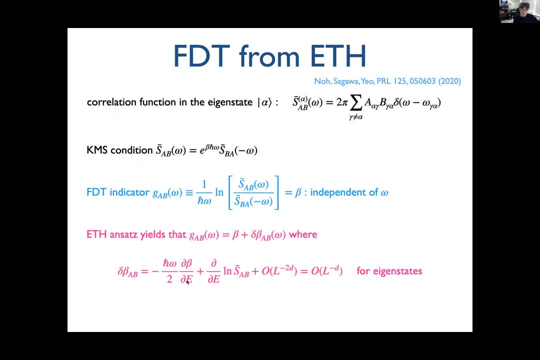 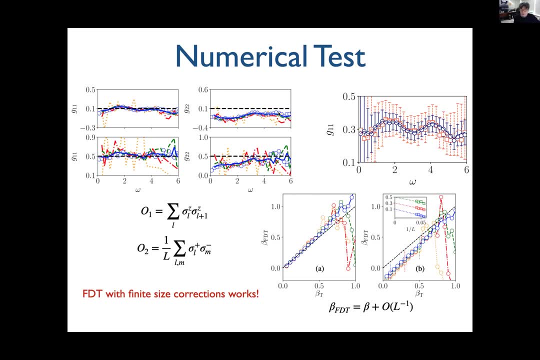 our, this finite size correction term. okay, So what that means? so you can see a symbol here, this blue symbol. okay, Blue symbol means the our prediction based on our finite size scaling series. okay, And this prediction is is almost indistinguishable with this numerical data. 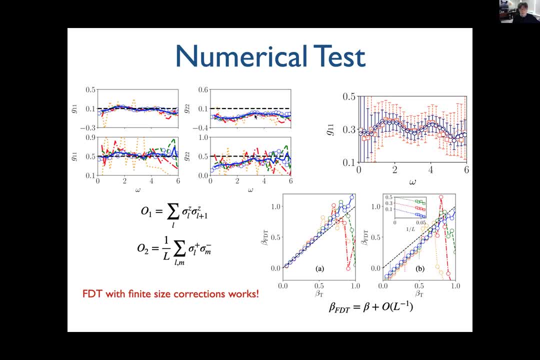 represented by a line. okay, So we expected all this fluctuation. fluctuation vanishes eventually in the thermodynamic limit. I mean the light, the long spin chain limit, okay, And we checked this behavior for five different observables. 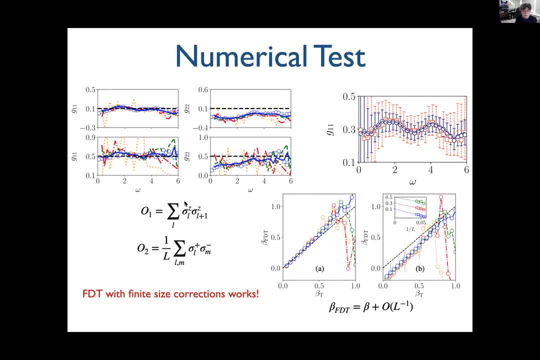 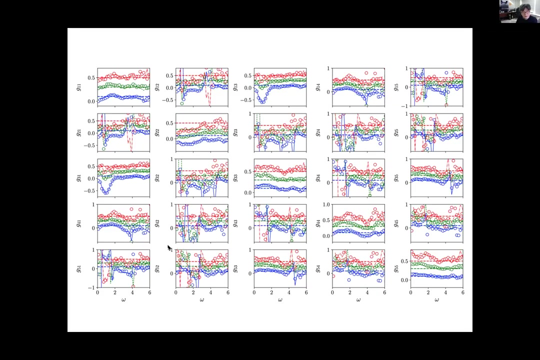 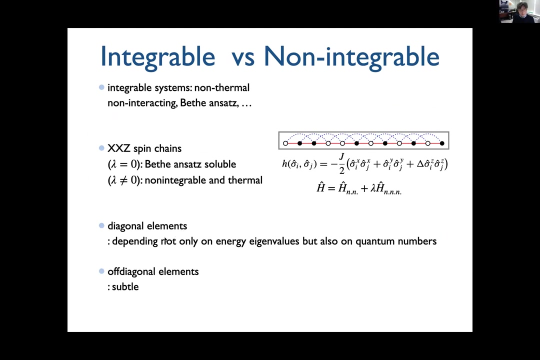 for example here for some nearest neighbor interaction and zero momentum distribution. and also we consider five different observables in total And in every case we check our final size scaling theory really consistent with the numerical data. okay, So actually I have some other parts. 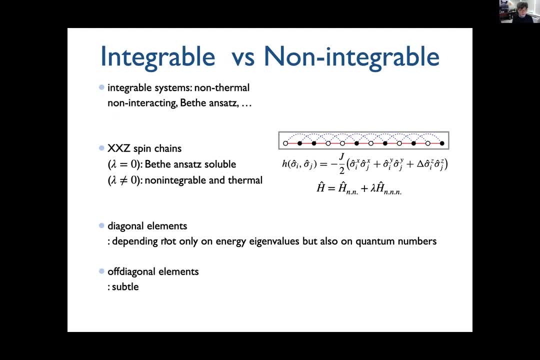 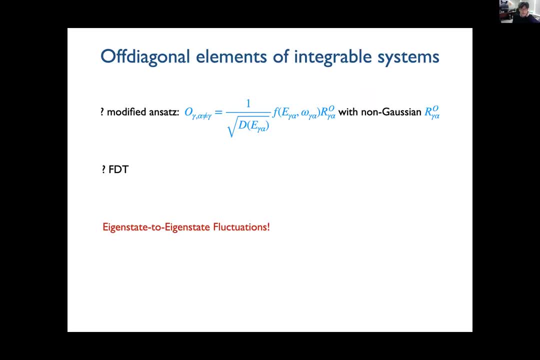 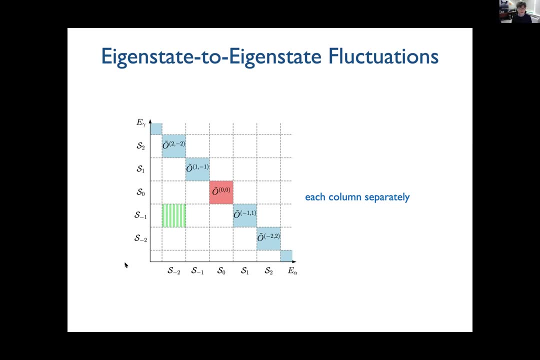 for the eigenstate to eigenstate fluctuations. but I think the time is up So let's see just okay. so I just show you the meaning, explain just the meaning of eigenstate to eigenstate fluctuation, okay, So. 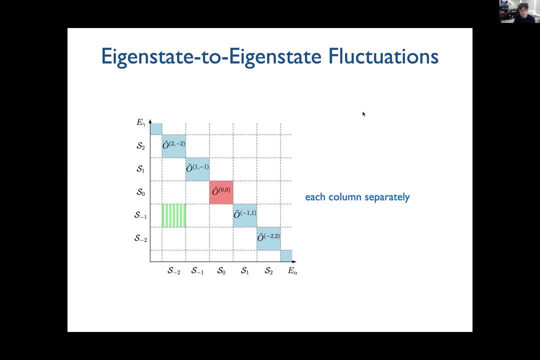 in the first part I wrote down some formal expression of the eigenstate thermalization hypothesis, and this hypothesis involves some matrix element. They should follow the random matrix statistics. okay, So people. so in order to check this random matrix behavior, 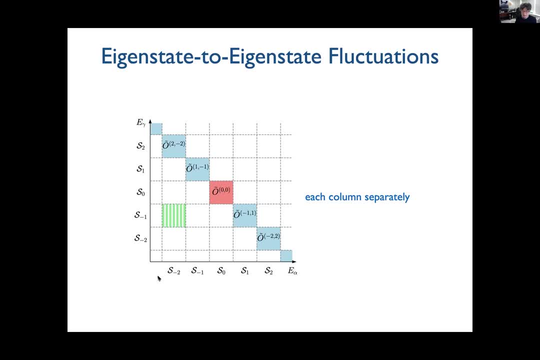 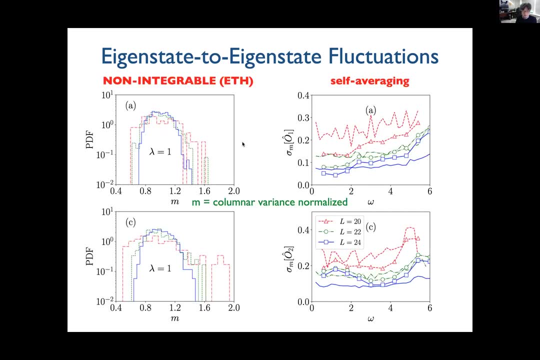 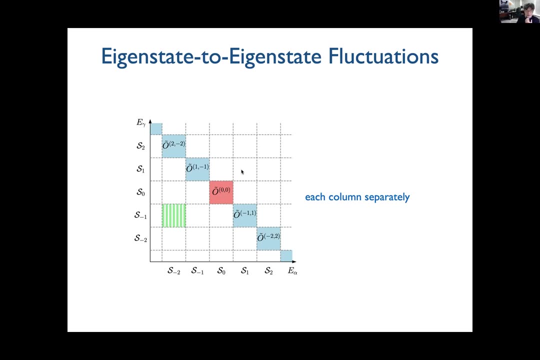 people usually diagonalize Hamiltonian and construct a matrix element. So this is the energy axis and this is another energy axis. So each point means some off diagonal matrix element: okay, diagonal matrix element- okay. So people usually consider this some small block or some massive. 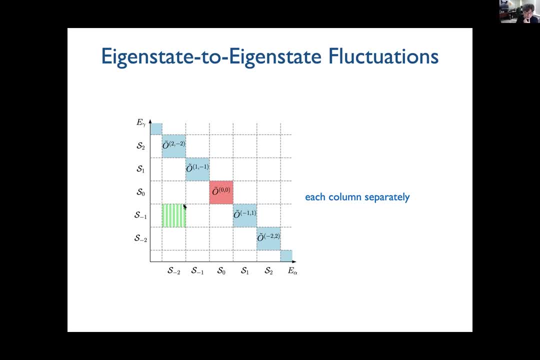 block and take all the off-diagonal elements within this block and then construct a histogram and compare this histogram with a Gaussian distribution or other theoretical predictions. okay, But, as I mentioned before, not every model obey the ETH. There are some exceptions, okay, For example, the integral of a system. Integral systems do not. 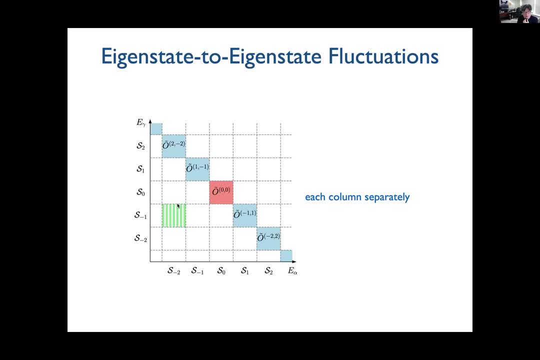 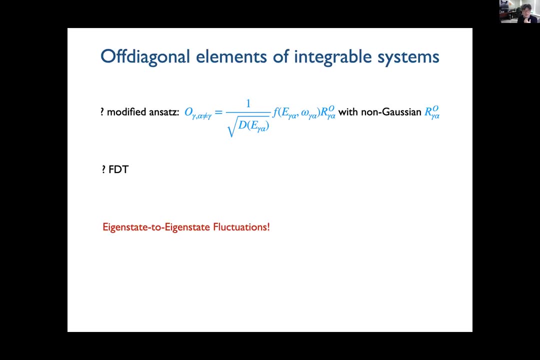 follow the ETH prediction, but nevertheless we can, I mean, investigate the statistical properties of off-diagonal elements, even for the integral of a system. okay, within this block. okay, You can. so this is, this is the numerical result. okay, For the. 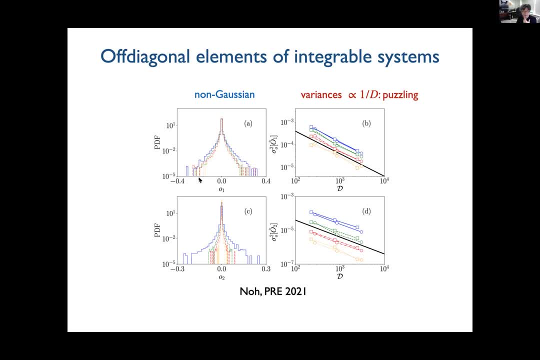 thermalized system we have a nice Gaussian distribution. okay. But in the integral system- I mean non-thermal integral system- they deviate from the Gaussian distributions. There is no theory for the shape of this distribution, but numerical distributions need a normal distribution to derive a. 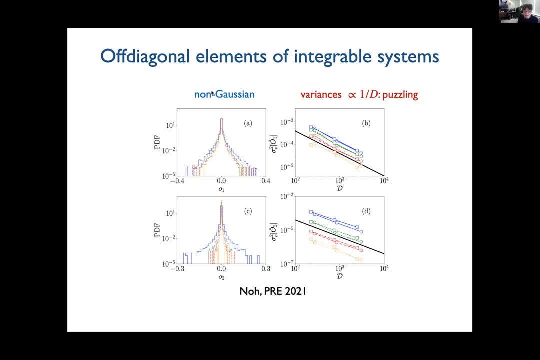 general Iceland. I mean the thermal system, But the point is that when I derive our FGT using the ETH, and that's the main ingredient, is this variance, not the distribution shape? okay, So here is some puzzle, because we know that interior systems do not obey the 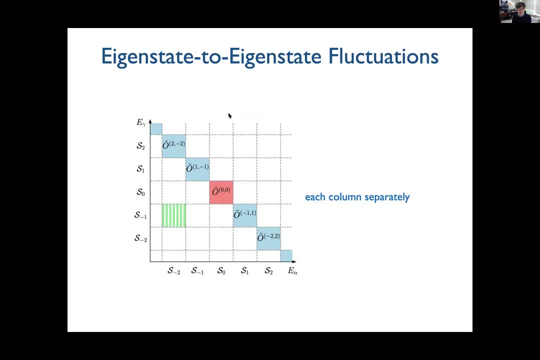 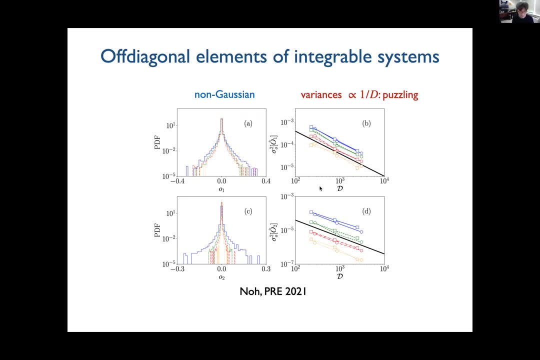 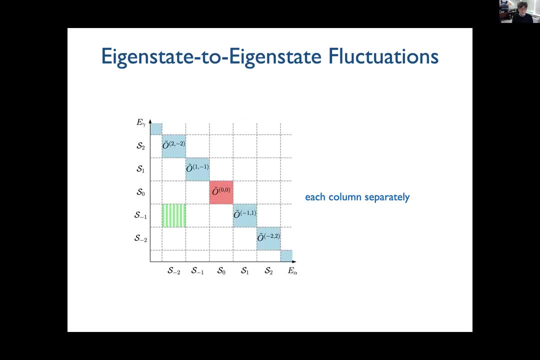 the fluctuation dissipation theorem, but still their variance is inversely proportional to the density of state. So it's kind of a puzzle in regard to the fluctuation dissipation issue. So my idea is that if you consider, if you look at the statistical property of element within this block, 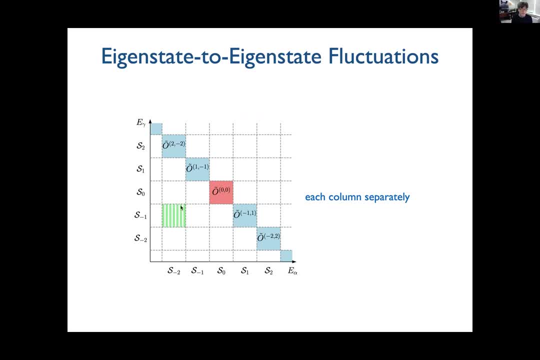 then you have some well-defined variance, even for integral system, but in the non-integral system. But if you look at the columnar distribution, the variance of each columnar element, okay, then we have some self-averaging behavior in the thermal system, But in the integral system. 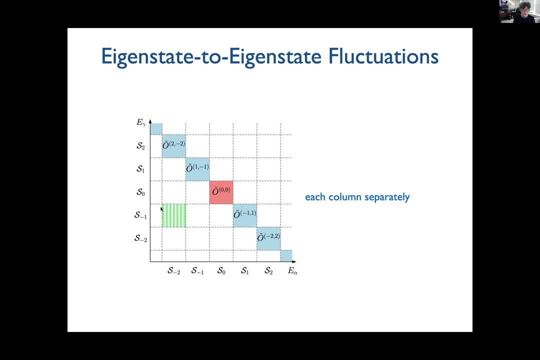 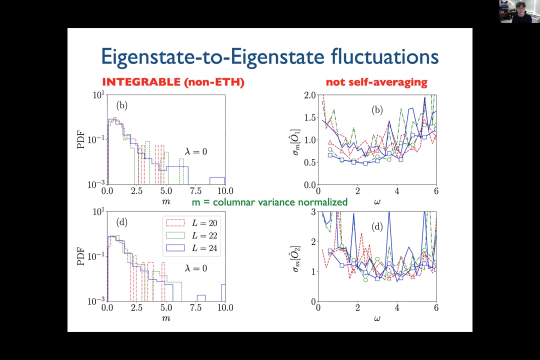 which is not thermal. we do not have the self-averaging property. okay, So there's some such a property I named eigenstate to eigenstate fluctuation, So that prevent the integral system from satisfying the fluctuation dissipation theory. That's the main message of the second part. okay, So this is the summary, and 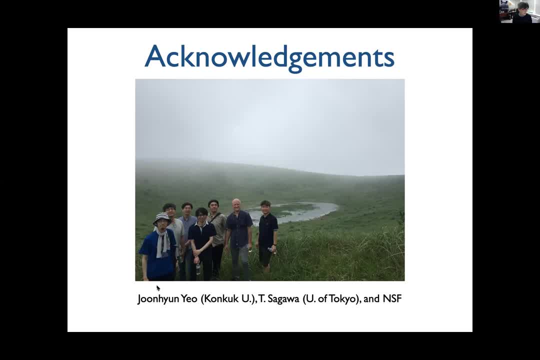 if this picture was taken into two years ago, 2019,. okay, I had, I organized a workshop in Jesu Island and actually my this was initiated in this excursion. okay, So it's me, and this is Takahiro Sagao of the University of Tokyo. 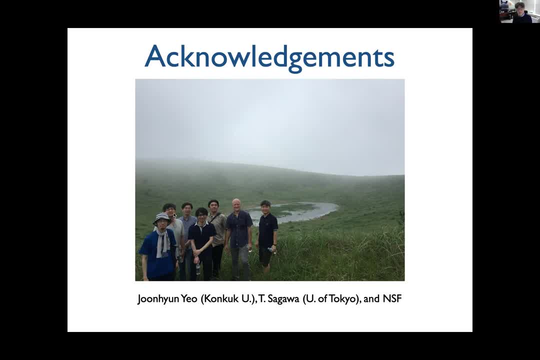 and this is Junhyun Yeo and the course of my PRN papers. So that's it. Thank you for your attention. Thank you very much. Thank you, Jae, for this exciting talk. So we are almost out of time, but maybe we can take one question. We already had quite a few. 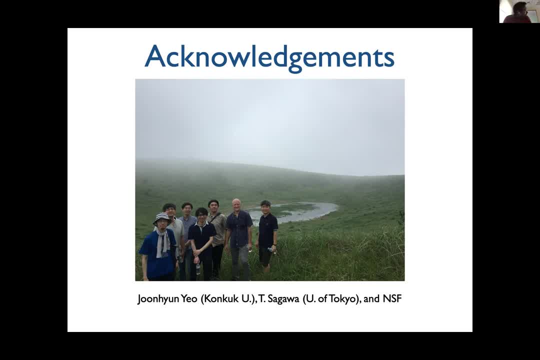 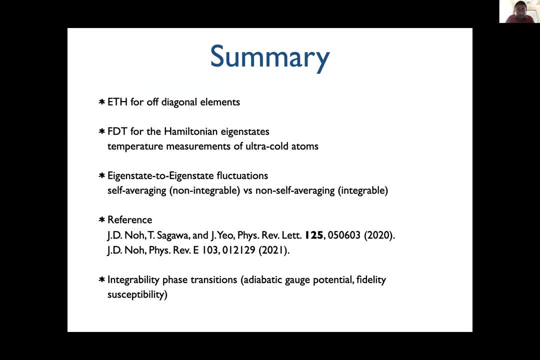 questions during the talk. So maybe one question and in the meantime, Gabriel, you can set up for the next talk. Maybe can I ask what you mean by integrable quantum system precisely. I mean every quantum system has with the eigenprojectors belonging to the Hamiltonian. 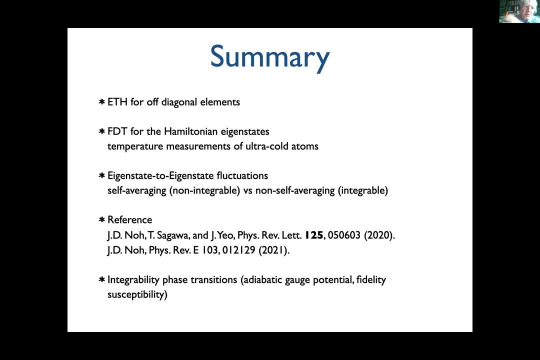 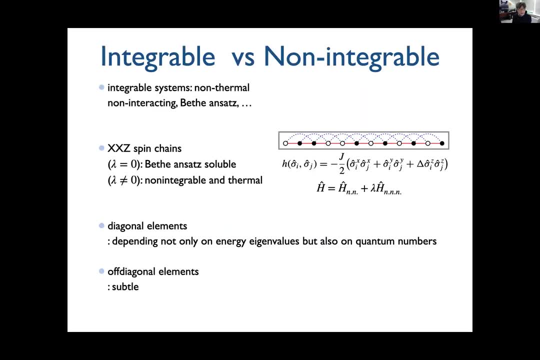 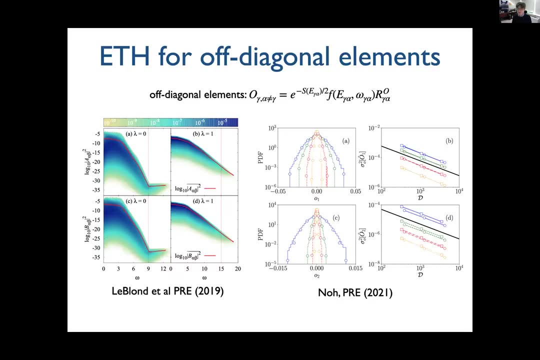 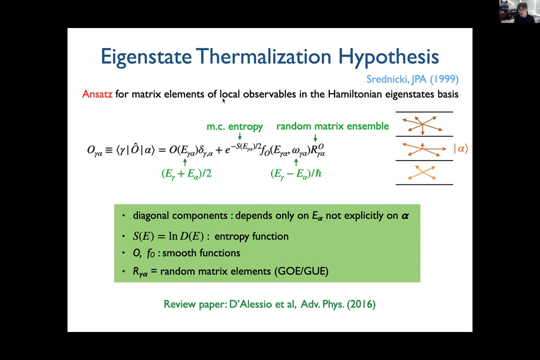 enough conserved quantities, so that cannot be the condition. Yes, okay, So unfortunately I do not have some formal, precise definition of integrable system. but actually this ETH is talking about some low-level observables. The eigenstate projector you mentioned is a really global quantity, so 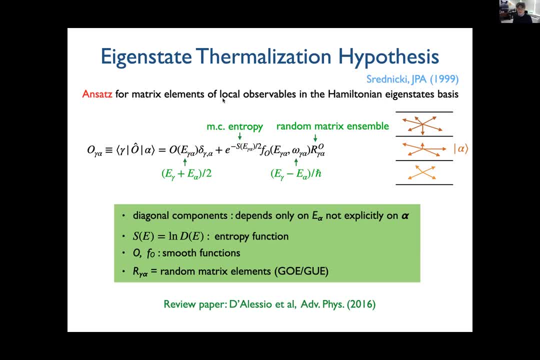 such a global quantity, we cannot say anything. See here. okay, So then actually this is not the real answer to your question. So actually I do not have some precise definition of integrability. so formally I can say that if you have some infinite number of 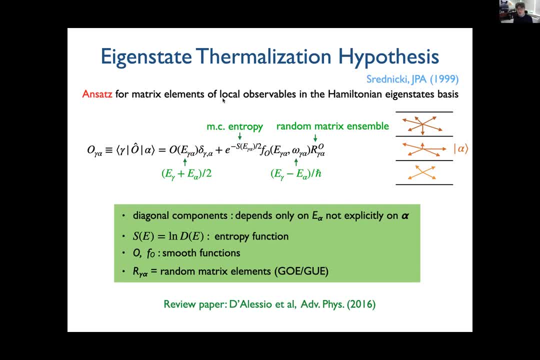 conserved. quantity, then quantity, then the system is said to be integral And there are some indicator of integrability. But I'm not sure whether that can. such an indicator or signature can be regarded as a definition of integrability. So in some sense, 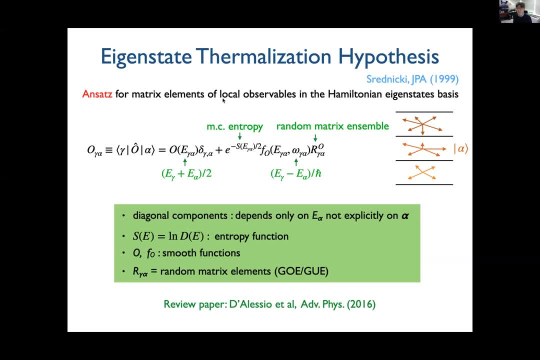 it's kind of operational definition. Okay, thank you, Jay. maybe I can ask one quick one last question. So is it okay if I say, for example, if ETH holds, then it immediately implies FDT will hold, or the reverse treatment Can I make? 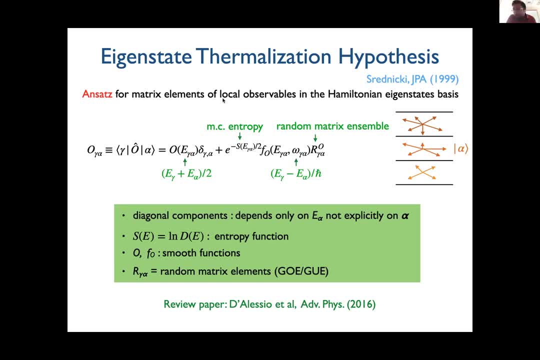 that, Yes, ETH implies FDT, FDT- Yes, Thank you. So okay, Mahbub has raised his hand so quickly. maybe one minute, One minute. I have only one query here that Ewald was talking about, the thermalization. So the results from this ETH and the 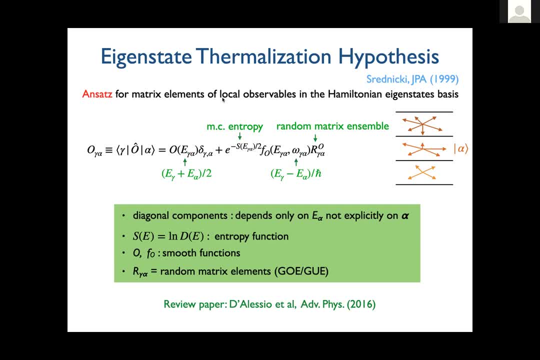 mean field. dynamics is equal or not ETH and mean field. Yeah, if I'm, if I do all those thermalization and get the result, and I'm doing the against it, a thermalization hypothesis- and do all the same calculations again.